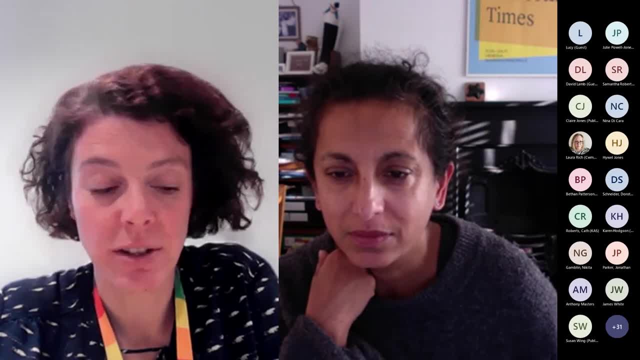 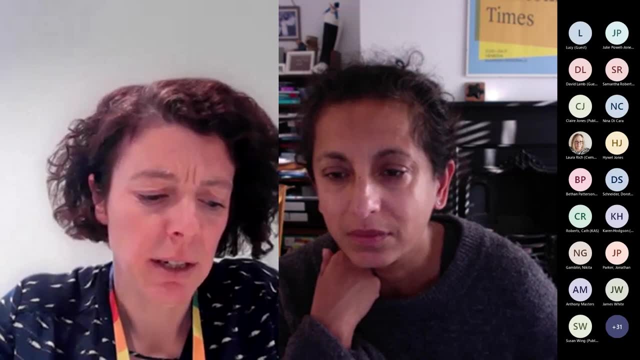 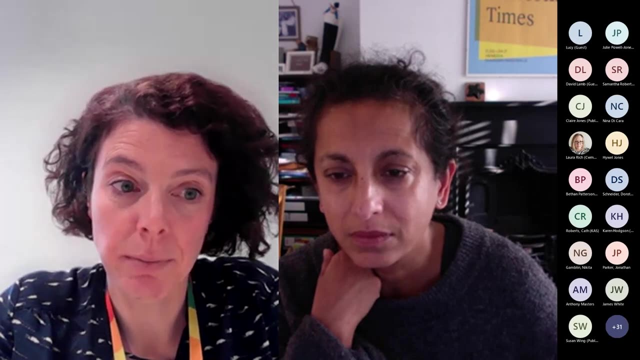 data science centre down there, Focus on suicide and self-harm research- really important areas in public health- and also the PI for the National Centre for Mental Health and the Wolfson Centre for young people's mental health, here based in Wales. So, Anne, over to you. 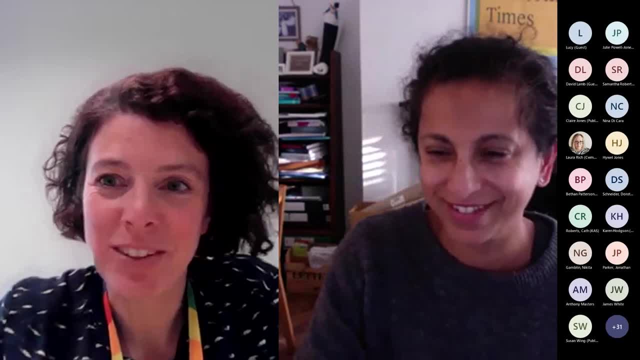 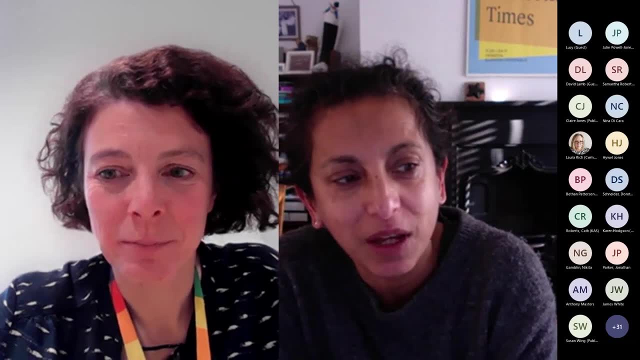 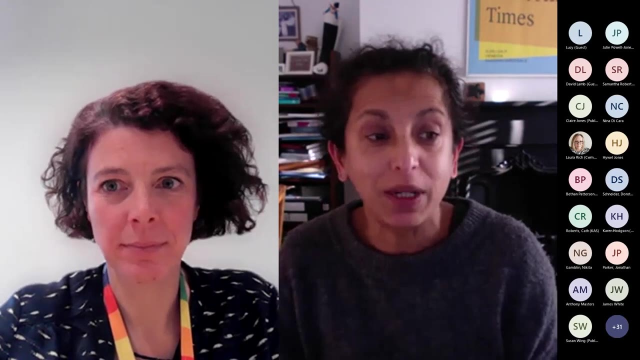 presentation on how do my feelings become numbers. So I'll hand it over. My background is: I started off life as a GP and then I did public health. so I worked in public health and now I have a split role, and I guess the reason I called 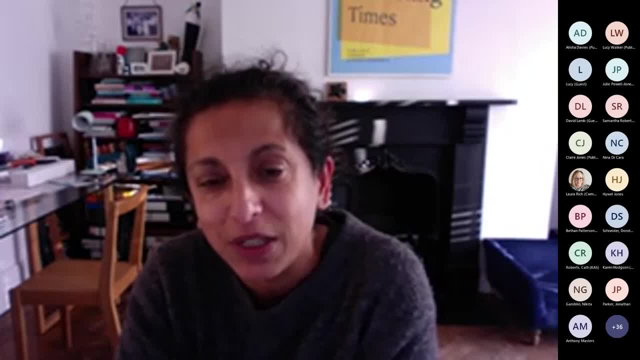 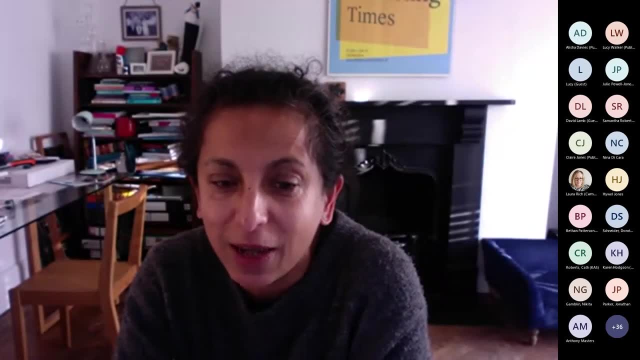 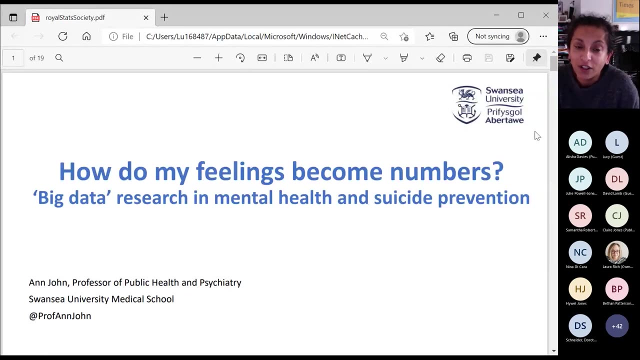 my talk, how do my feelings become? numbers is because I think one of the challenges that there's been in terms of statistics and epidemiology is communication Of what are often complex analyses and graphs to people, and particularly in the field that I work in, where it's sort of children, young people's mental health and suicide and self-harm prevention. 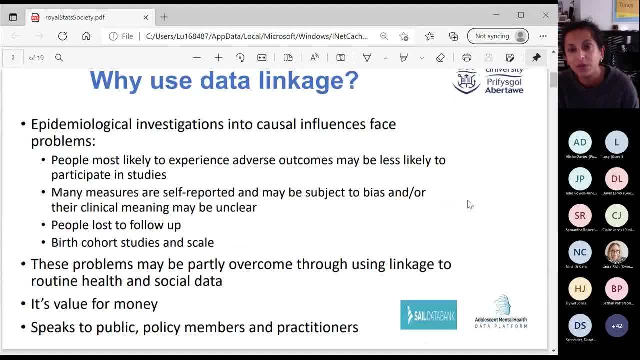 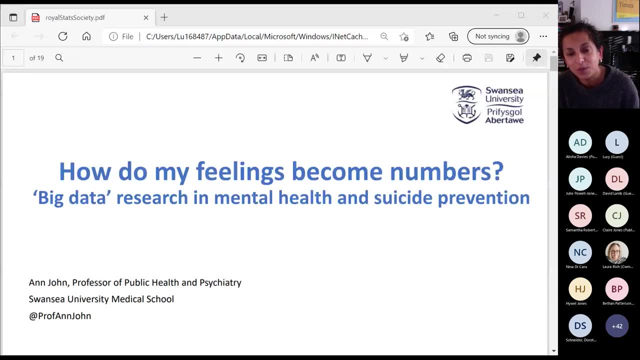 You can often see, you can often seem like you're being quite cold in the way that you talk about data, and I guess there was one. there was one presentation I did at a science festival and some of the young people in the audience were sort of quite challenged by the fact. 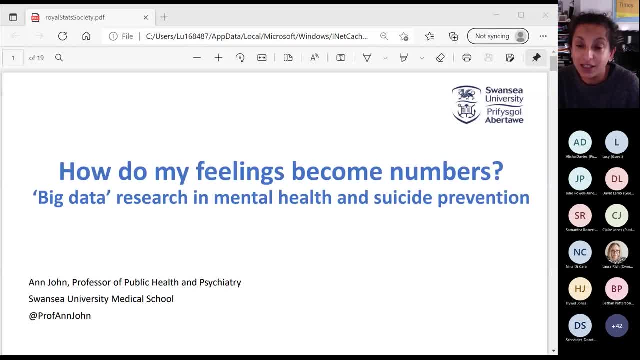 that we were using their health data to assess their mental health, and one of them actually said to me: how do my feelings become numbers? and you know, by the end of talking it was clear what we were doing, but I think that there is a communications issue. So next slide. 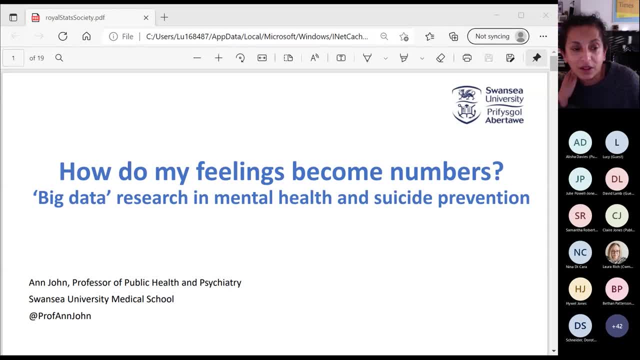 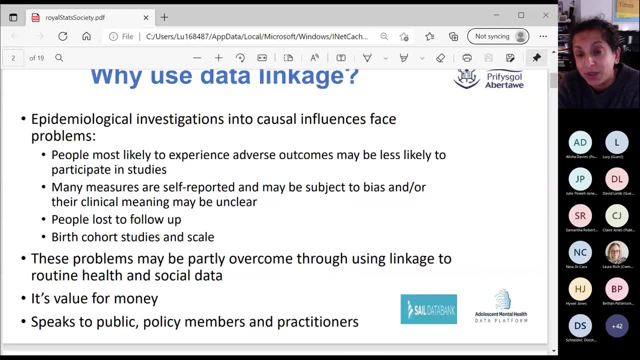 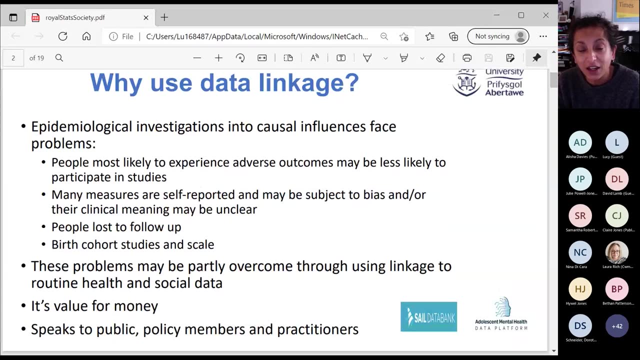 Um so. so I work a lot in um, the Sale Data Bank, predominantly on data linkage, so where we link at an individual level across lots of different um data sets. Now the reason I've sort of ended up after quite a convoluted career doing my work there is that when you think about lots of cohort- 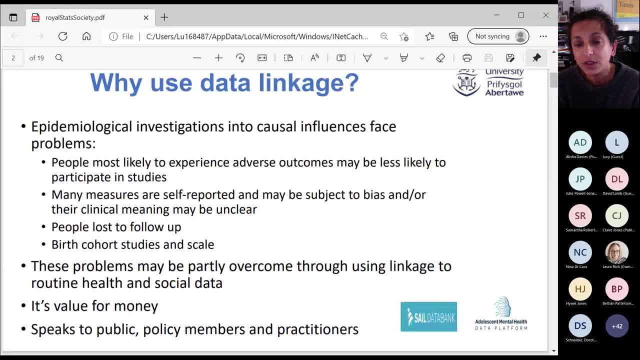 studies and questionnaires- Yeah, Those you know. so questionnaires that go into schools, those who are the most unwell in terms of mental health conditions are often the least likely to participate in those studies. Now, we don't find that to be the case for questionnaires that come to people's houses. 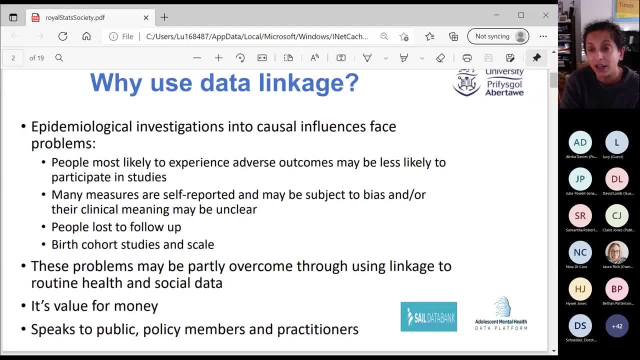 There's really mixed evidence about whether those with more severe mental health problems answer those or not, But in schools there is evidence that young people just aren't there on the days that they're being asked to do things that are unusual, So those with the most adverse outcomes aren't there. 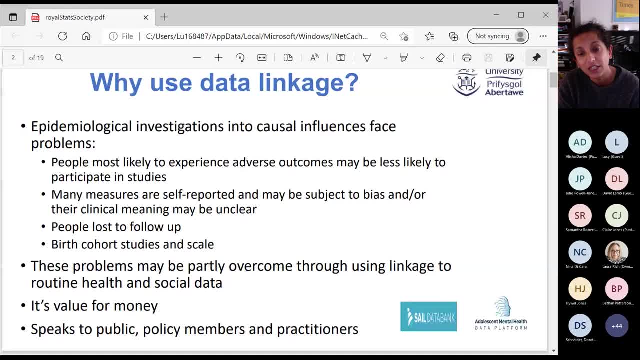 A lot of the measures in a lot of the data that we work with are self-reported. So when you're talking about a term that is so much in common usage, unless you're using validated scale, they're quite subject to bias. And even when we do use validated scales, like GHQ-12, which I'll talk about later- there's often debate within the field. 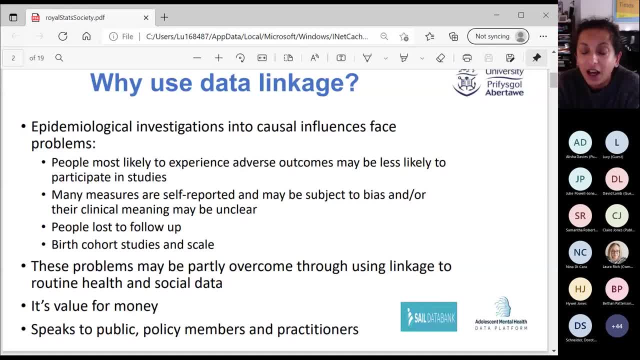 You know the work I'm going to present later. I was asked by a psychiatrist, you know, do you really think that these sorts of well-being scores reflect mental health? So you know there's difficulties with that And when you look at sort of like the birth cohort studies that run for many years, people are often lost to follow up. 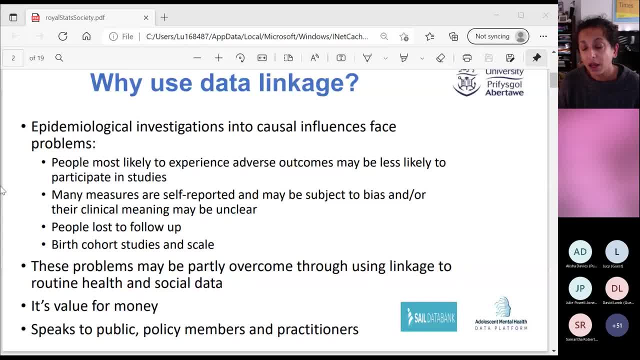 So you know, when you think about your original cohort and the people who are answering your surveys in their- you know, 20s, often the people that I would be most interested in are gone And there's something to be said with, like, you can't measure what isn't there, however well designed. 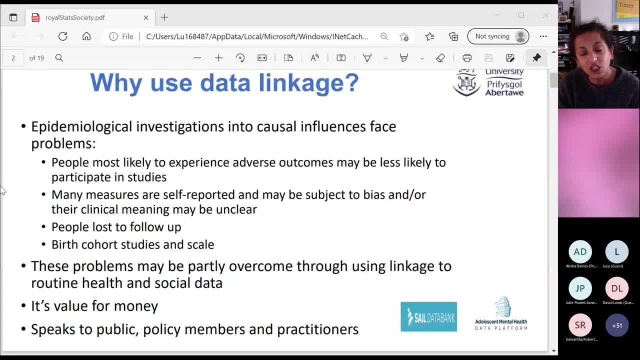 Your cohort is. And then I guess the other issue with some of the with some probability sample surveys in both cohort studies is that for some of the things like schizophrenia and bipolar disorder, so rarer outcomes, we just don't get the numbers. 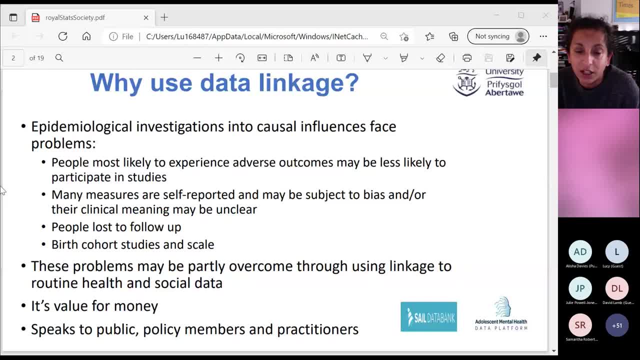 So recently we did a in the Adult Psychiatric Mobility Survey. we did a piece of work on problem gambling and suicide And you know, and we found significant findings, But I was really aware that it was actually based on 49 people. 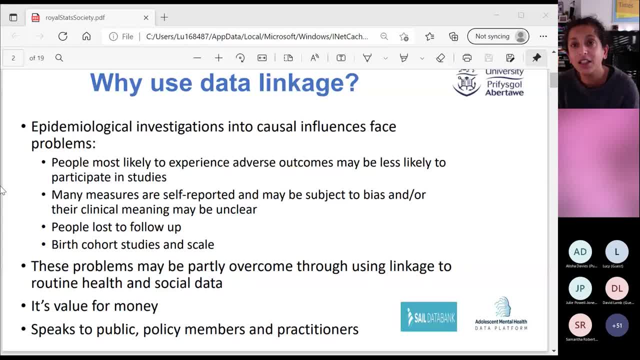 So some of those problems are partly overcome by using, you know, large scale, routine health and social care data at a population level. That sort of secondary analysis is good value for money. And then I think, most importantly, it speaks. If you phrase it in the right way, it really speaks to. 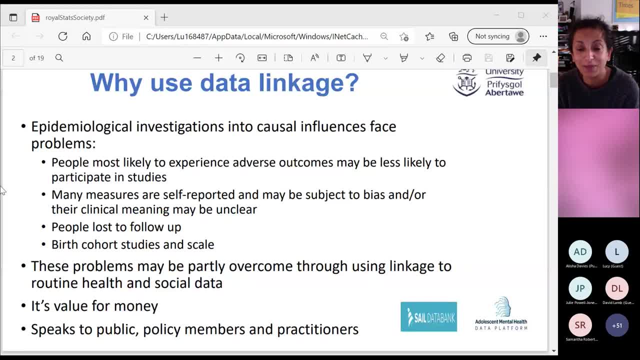 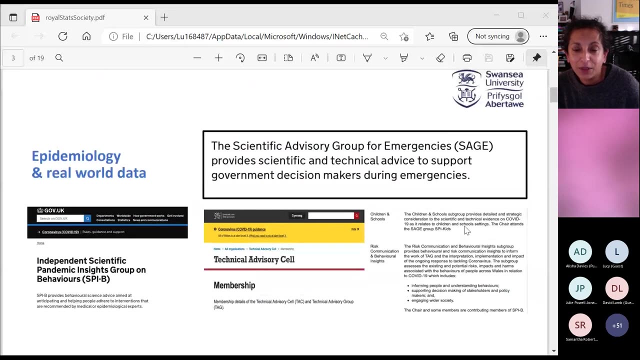 People and policy, not policy members, policy makers and practitioners. So you, you're really demonstrating things that are in the real world. Next slide, please. So I guess you know a few. Two years ago, when I said that I was an epidemiologist, no one knew what that was. 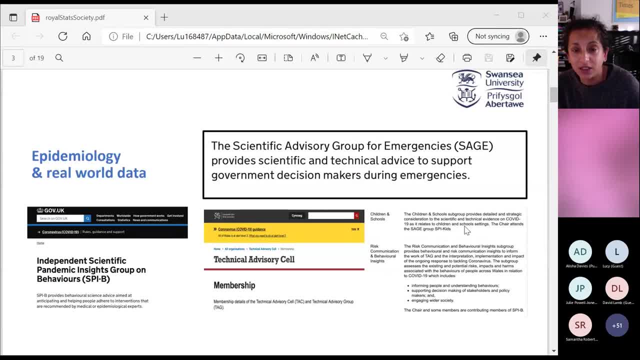 And if I put a graph Up in front of, in front of some audiences, they would, their eyes would glaze over. I think Covid has changed a lot of that. Everyone knows what an epidemiologist is. People have been looking at graphs every week. 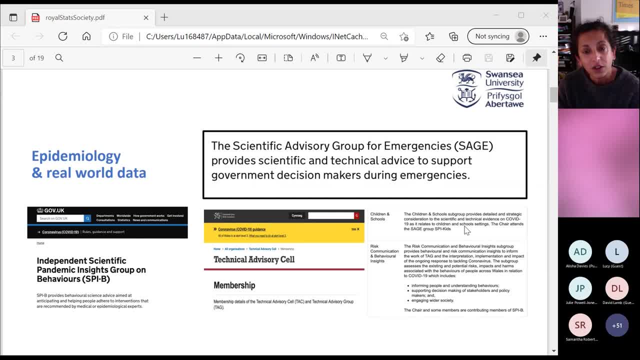 And I think one of the things over the last two years is is I found myself. I sit on SAGE. I co-chair a subgroup of SAGE, Spy B. I've sat on the Welsh Government advisory group, TAG, And also chair one of its subgroups and sit on its children and schools subgroup. 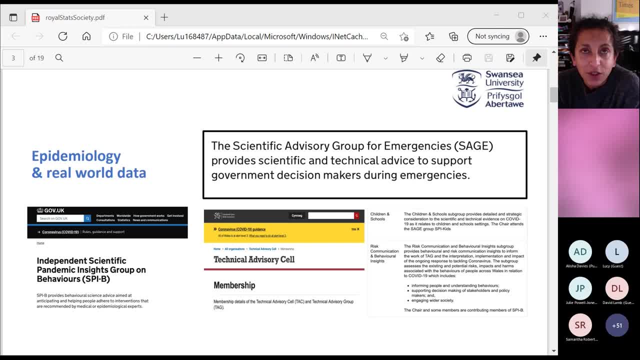 And I guess there It's both a challenge and an opportunity. So all the skills that we, you know, we've all developed in terms of thinking about what sorts of analyses we do, what are the limitations and challenges of it, mean that you can take those skill sets into those sorts of government advisory groups. 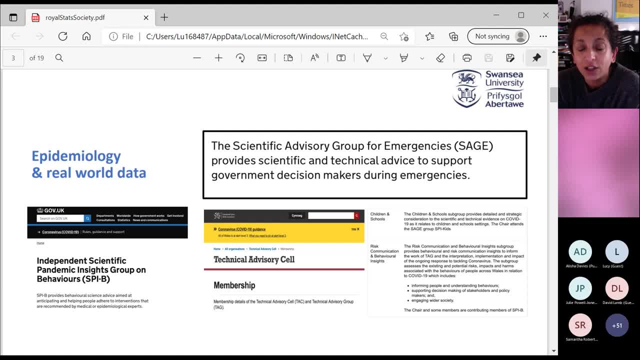 It's a challenge, It's an opportunity- roles and interpret the rapidly emerging evidence that is being placed in front of them. So you know, in some ways I think all the challenges of statistics became the reason why I ended up in the advisory roles that I did. Next slide please. 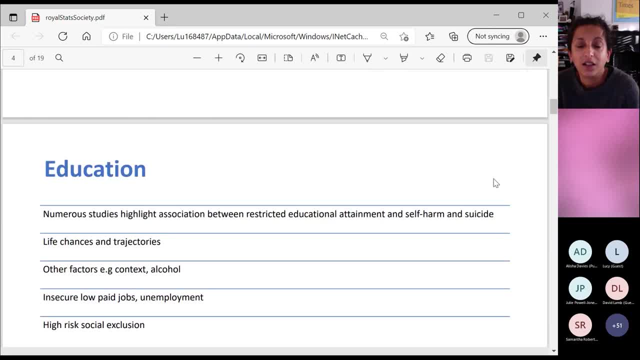 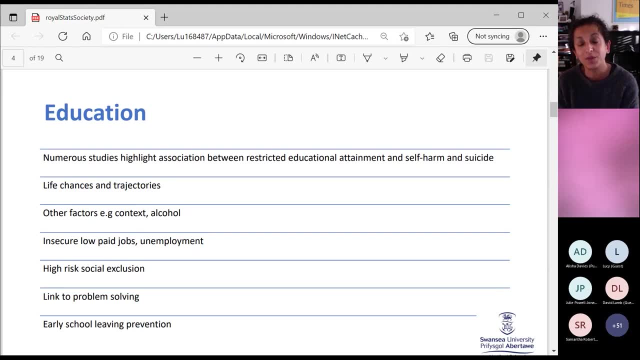 So I guess the first piece of work that I wanted to talk to you about was something that's going to be published tonight. so it's it's hot off the press and it's to do with mental health problems and education. So there's lots of studies out there that highlight the association between 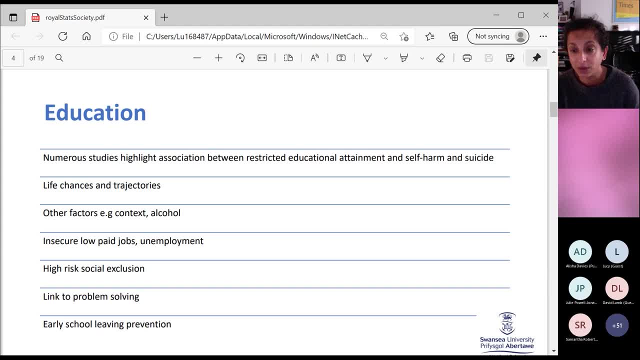 poor educational attainment and self-harm and suicide and also mental health problems. now there's lots of reasons why we think those problems happen. you know, if you, if, if you don't do reasonably well in school, it has impacts on your life chances and trajectories. it's a bi-directional relationship um lots of young. 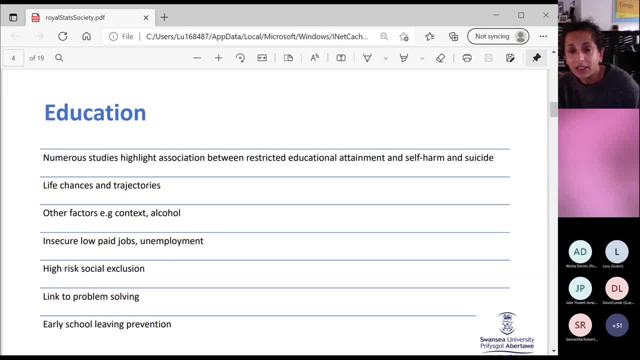 people who have problems and adverse childhood experiences when they're younger will pick up more as they become older. uh, people go into more low-paid, insecure employment or unemployment. um, and higher levels of education are linked to higher levels of problem solving skills and those? um that's one of the risk factors for suicide and self-harm. um and so so there's lots. 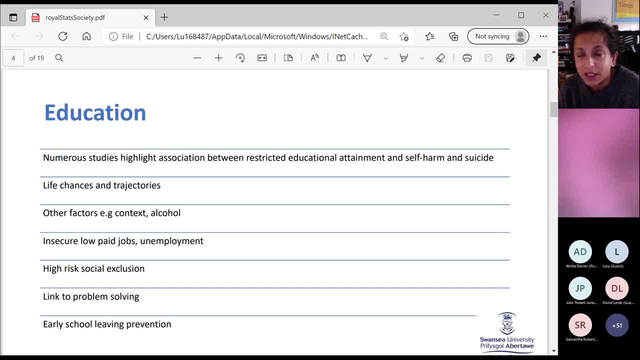 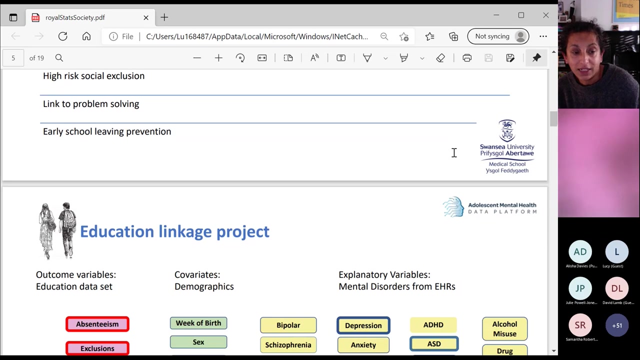 of work done about attendance, but some of that has tipped into um being very much focused on rewarding children who reach 100 attendance, and sometimes there can be very good reasons for not reaching 100 attendance next slide. so what we did was within the sale data bank and i- and i know, having looked at at some of the names- 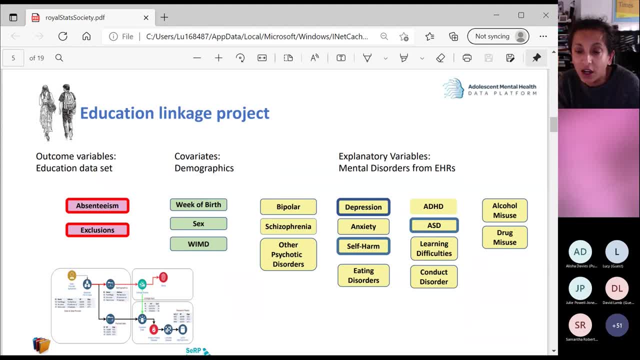 um of those of you that are here that some of you have worked within the sale data bank but haven't. sale um has a split file anonymization approach. so if there's a data set, say, like the general practice data set, the clinical um information is separated from the identifiable. 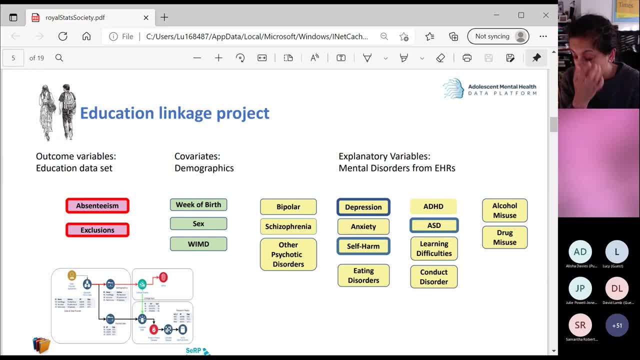 information that goes to a trusted third party, which is digital health and care, wales in this case, and it's given what we call an out, so an anonymized linkage field, now that individual in all states of the world has a split file anonymization approach. so if there's a data set, 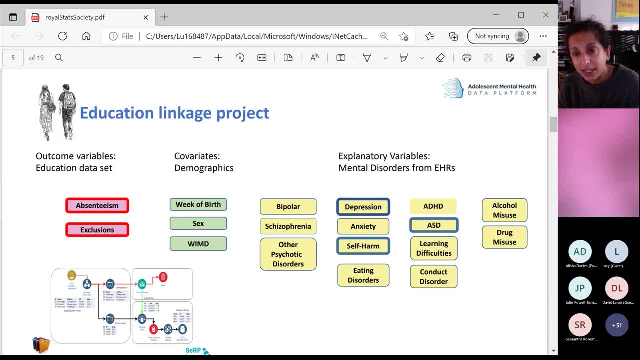 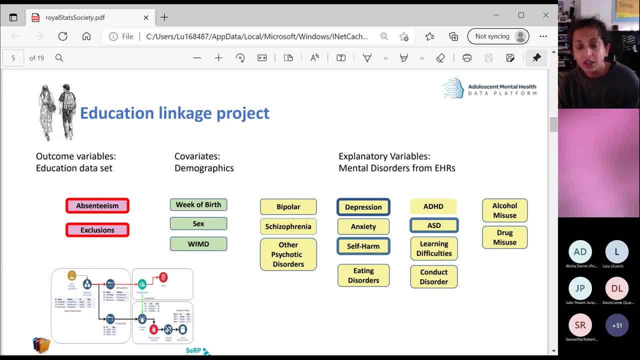 are five. identifying criteria are generally the same, so you can basically find that individual within each of those data sets. so in this piece of work we took the education data set generated um through local authorities and held by welsh government, and looked at levels of absence and exclusion, and then we took an array of different mental disorders, because there's lots. 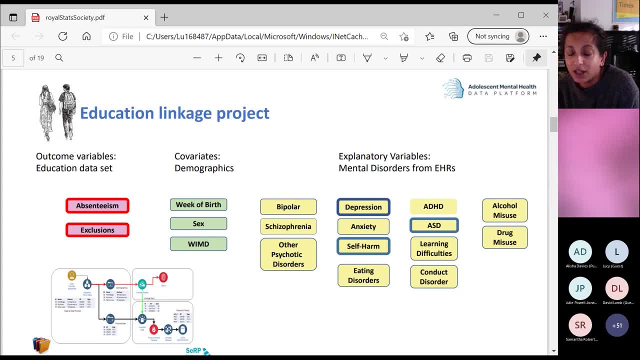 of theories out there about, um, what sort of mental health problems are associated with absences and exclusions, and i guess one of the things i said about the results of this study is it's sort of not rocket, rocket science, because unsurprisingly, we found that across the board. so 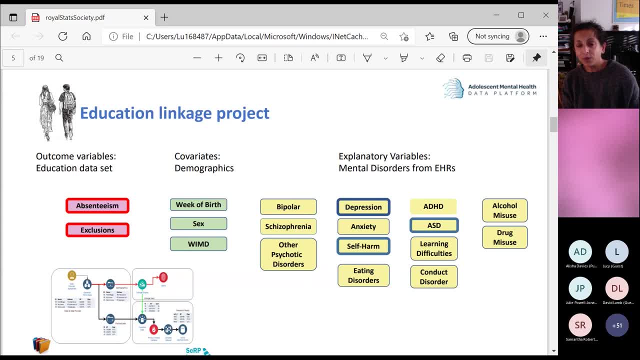 almost trans. diagnostically, mental health problems were associated with being absent and being excluded, and so so we're not doing anything that you know. we have a hypothesis i would have been. you would have not had to knock me over if we hadn't- um, we haven't proved it, but uh, the thing about this sort of work is that it provides the 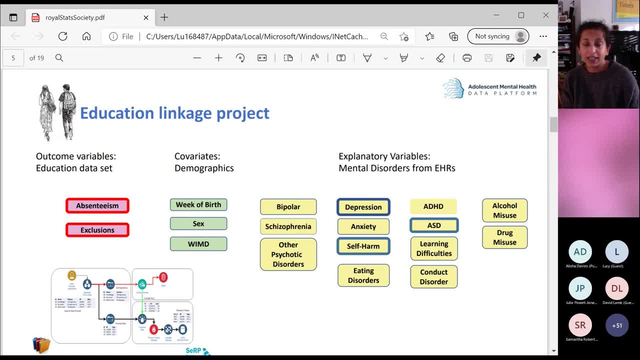 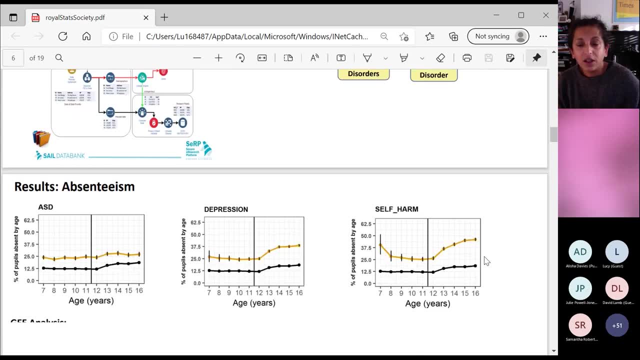 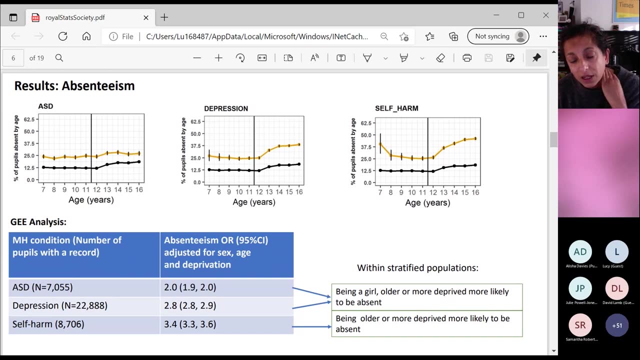 evidence and the scale with which people can take action. next slide, please. so what we found was that, um, unsurprisingly, across all those disorders, there was- uh, you know, young people who self-harmed were were almost three times as likely to be absent from school. now, there was an increase in absences. 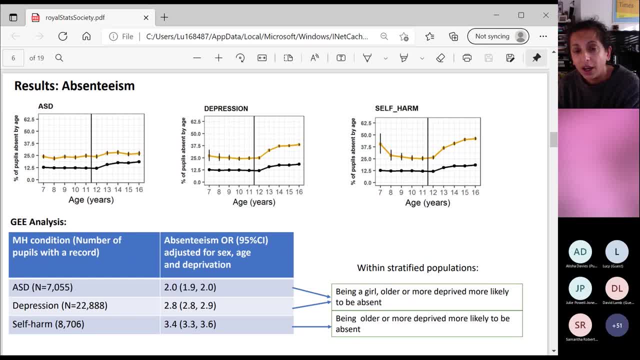 and exclusions across the board, um, in older age groups, so sort of 14, 15, 16, and we think that's about the fact that at those age ages parents start to have less influence over whether a young person goes to school or not, and one of the other things we did that 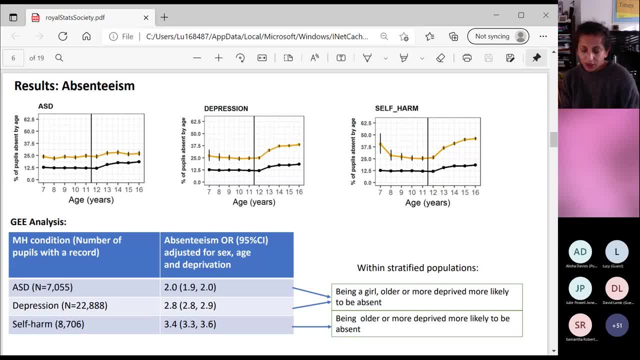 i meant to say was so. there's lots of delays in diagnoses of children with mental disorders. now we know about three-quarters of them start before young people reach the age of 24.. um, now, with that, what that means is, is that for some, so like schizophrenia, bipolar disorder, a very 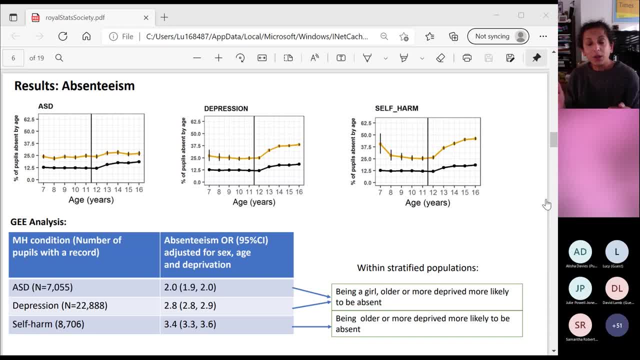 serious disorder. it was awful for young children. yeah, disorder are very unlikely to be diagnosed prior to the early 20s, but there are impacts in terms of, you know, cognitions and emotion that mean that a lot of there will be sort of pre-diagnostic effects in schools, so people will be feeling the impacts of their conditions well before their. 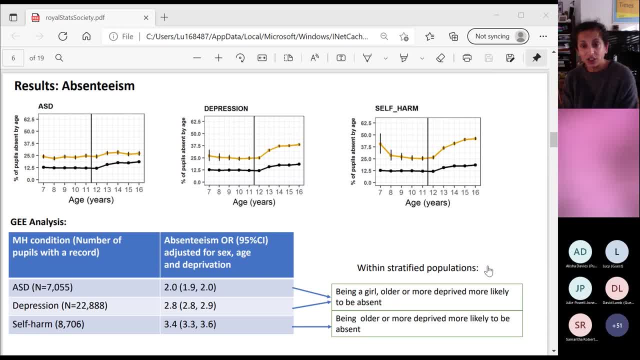 diagnosis. so we looked at- although we looked at- education up to the age of 16 in order to address that challenge of knowing that people get diagnosed at all sorts of different ages for different reasons. like you know, you've got to go to your GP. that's one barrier. you've got to your 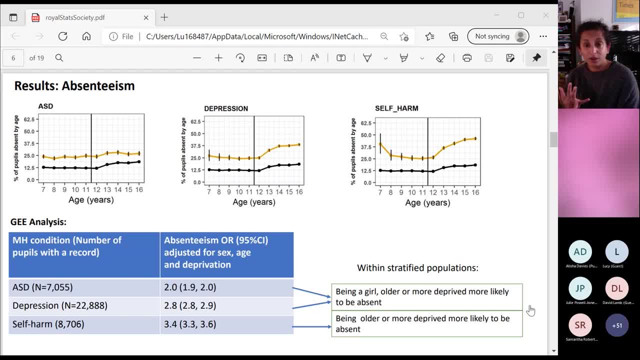 GP has to recognize that there's a problem. but even if they recognize it, they then have to record it, and so, to to allow for the timelines across some of those issues, we we measured our diagnoses up to the age of 24.. We also, for neurodevelopmental disorders, took any diagnoses from birth, because those tend to. 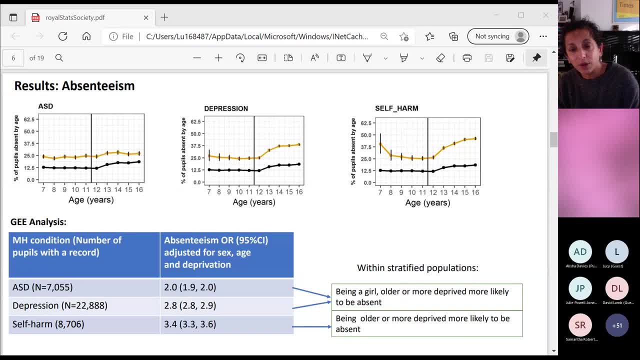 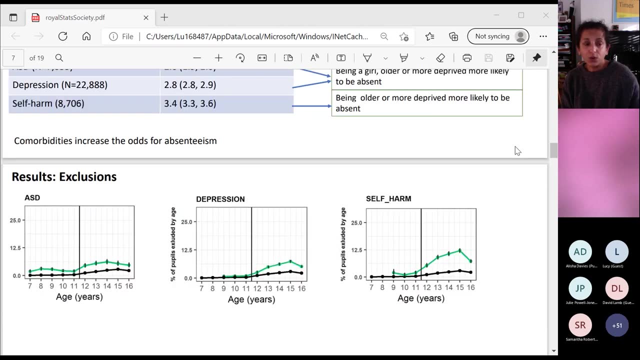 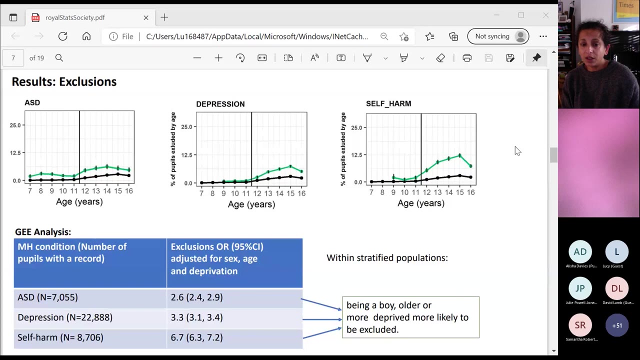 be diagnosed when people are younger, whereas things like depression and anxiety it tends to be when young people are slightly older. Next slide, please. So we saw very similar things for levels of exclusion, except this time the odds ratios are much higher. so a young person who self-harms is almost seven times as likely to be excluded. 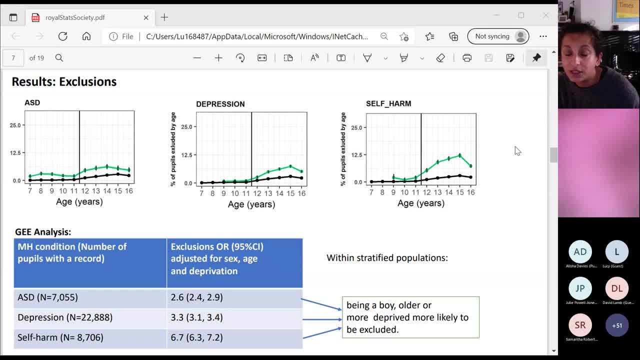 in school, from school, than their, their peers who don't self-harm. Now the impact of those sorts of exclusions. you know, across most of the western world there is a there's a push not to exclude young people, but I guess what this sort of work demonstrates can demonstrate really clearly. 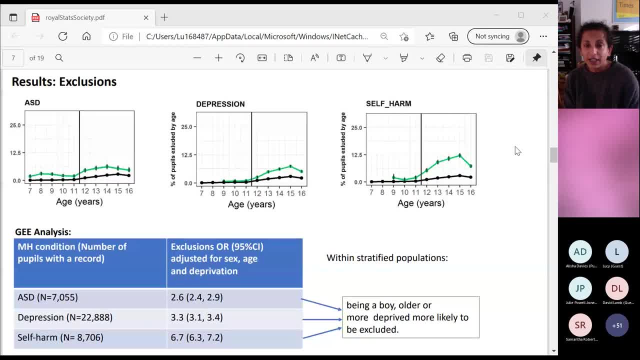 I don't know if we will yet- is how clear the relationship is between mental health problems and absences and exclusion, and that can that has the potential to change the story in terms of saying that young people who are excluded from school are not excluded from school. So we know that. you know, in terms ofulsions and stuff like that, but because of the ease of exclusion, people do have very strong health problems and I think we can really see that and I think that's what we're really looking for from the point and going to the next slide. To the next slide, please. 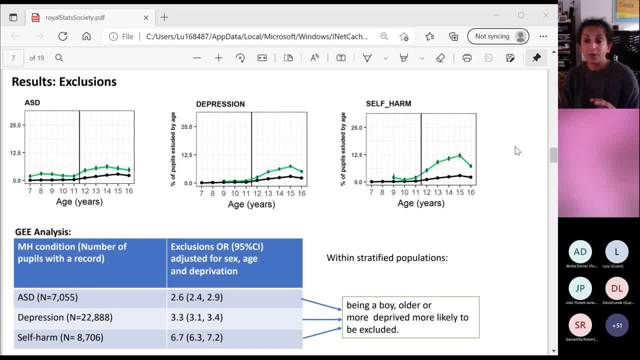 excluded and absent are vulnerable rather than it's about behaviour, And I guess one of the things we said in this piece of work was that there's a real- you know, we collect this data routinely- absences and exclusions- So there is a real opportunity to potentially identify young. 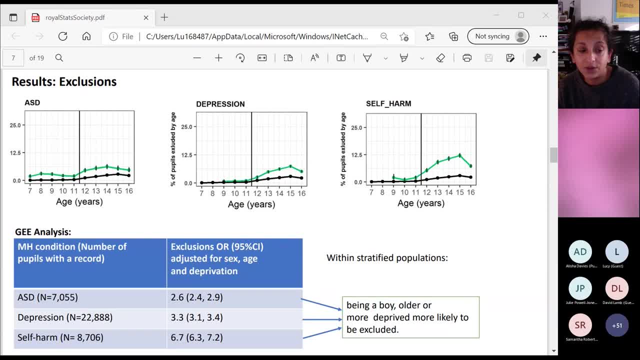 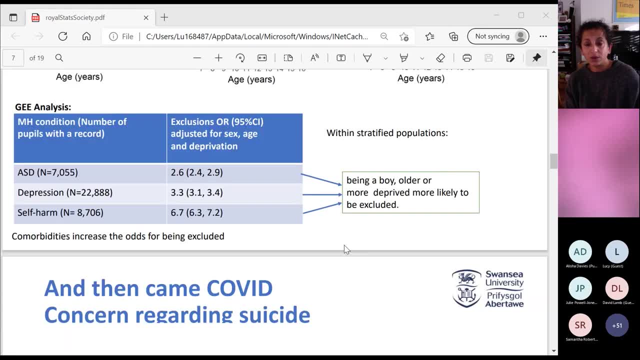 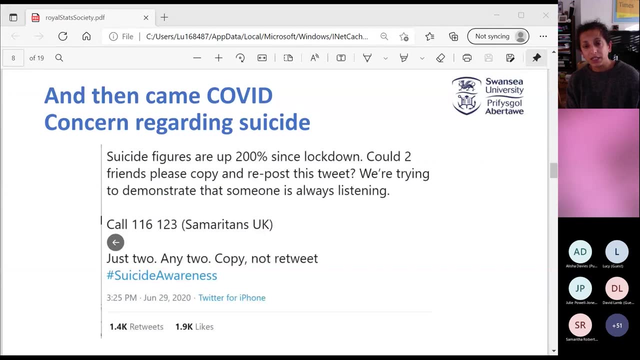 people who are in need of support at an earlier stage. Next slide. So I'm going to talk about some of the suicide work that we did following COVID. So some of the issues around suicide data is that all unexpected deaths- so those and suicide counts as one of those- have to have a coroner's. 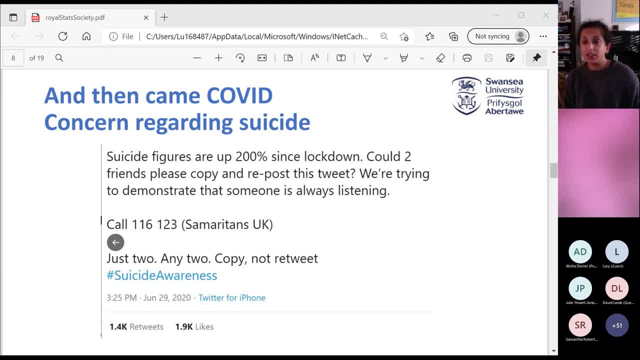 inquest Now. so we usually get an ONS bulletin annually- So many, so usually the stats we're working with are at least a year out of date. Now, during COVID, there was a lot of concern that suicide rates would increase. Next slide please, And some of those concerns were very 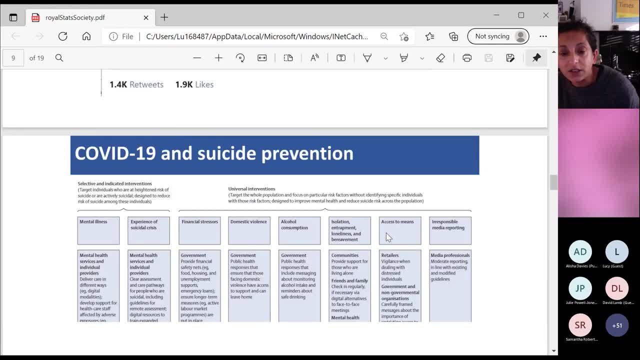 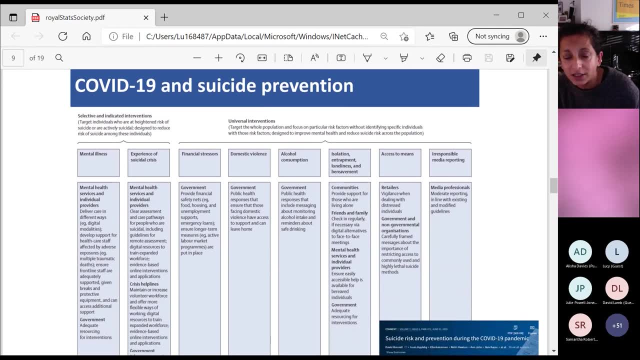 legitimate. So I sit on the steering committee of an international collaboration and we published an editorial early on and we highlighted things like you know: sets of loneliness and isolation during lockdown, People's exposure to domestic violence because they were because of stay-at-home orders. 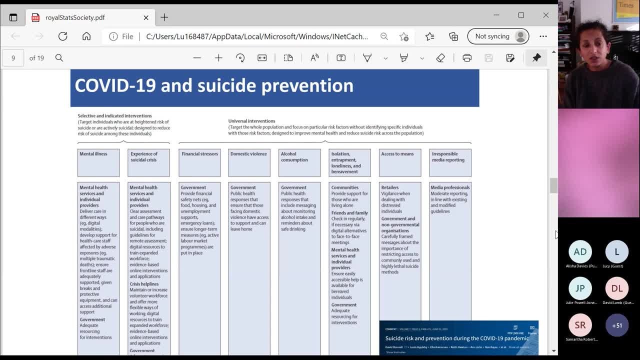 financial stresses. So those concerns were not unfounded. However, one thing we do know is that when people report a lot that suicide increases has increased or talk about methods, it can make vulnerable people more vulnerable. So you know we. 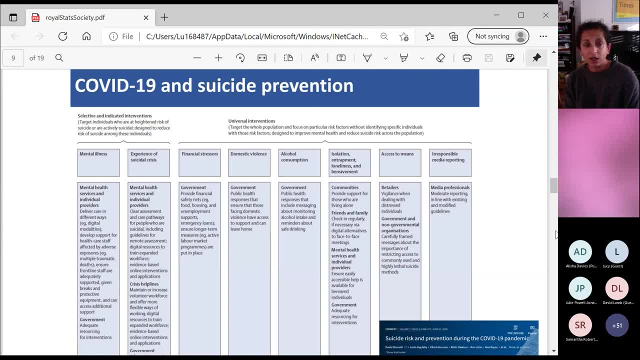 had. we didn't really in Wales we don't have a real-time surveillance system. In England there weren't many, And so it was really about how. the challenge was was about having timely data to answer the uncertainty of these questions. So next slide. So what we did was a whole bunch. 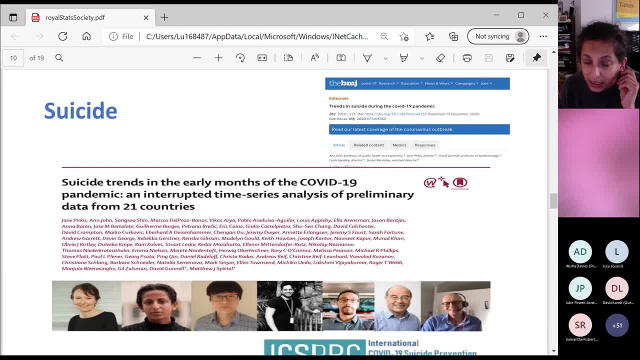 of us, led by Jane Perkis in Melbourne, but with you know, we didn't have a real-time surveillance system. So what we did was we set up an international collaboration. So we had, we set up an international collaboration with David Gunnell- myself in Swansea, and David. 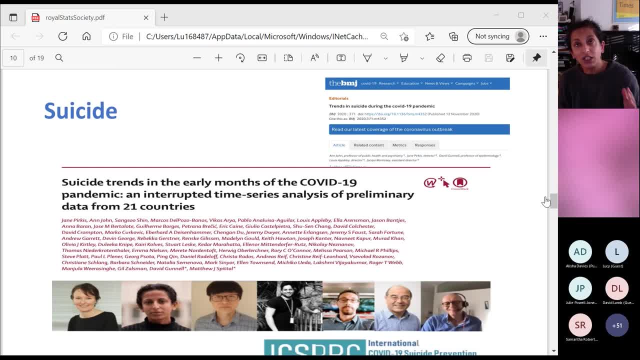 Gunnell in Bristol. We, through the international collaboration, basically set about. it all sounds very easy, but I don't think we could have done it if we didn't have the trusted research environment set up. So we basically contacted people from around the world and asked them for their suicide data. 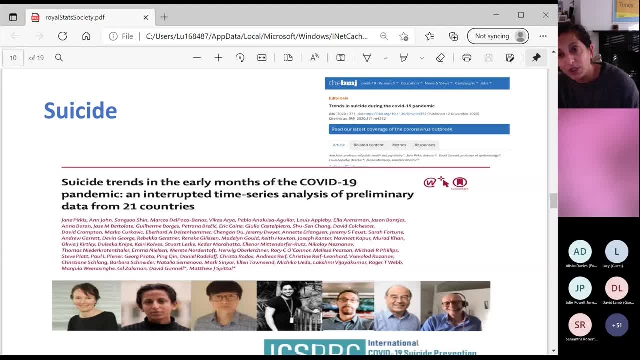 So we basically contacted people from around the world and asked them for their suicide data And we published a paper. and we published it at a time when people absolutely did not know what was happening with suicides and where there was a lot of talk that had been increased. 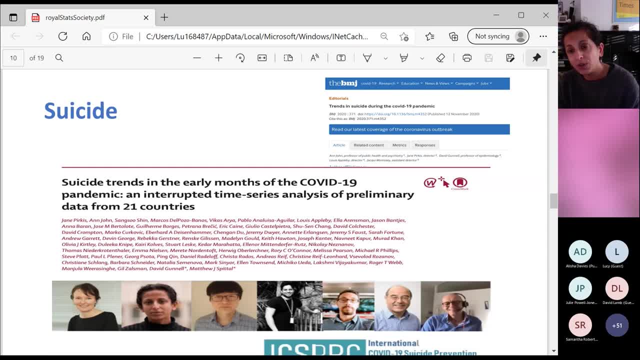 And that was tied in to all the anti-lockdown movements. So increasing suicide rates was very much part of that anti-COVID measures movement. So it was very vociferous on Twitter And some of us had, you know, had some quite challenging Twitter exchanges with people. 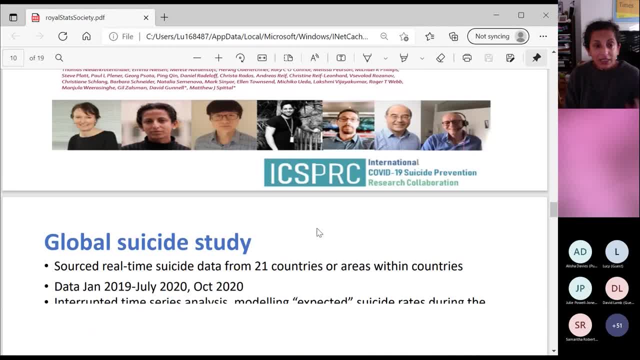 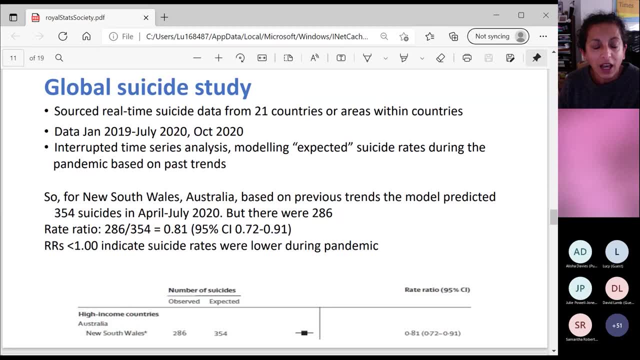 Next slide. So we basically sourced real-time suicide data from January 2019, because we wanted pre-pandemic trends, And up to July 2020, but we also had some from October And didn't interrupt a time-series analysis. They're comparing, observing and very quicklyP tungesting real-time suicide data. data, So comparing observed stunts and veteran deaths in the year 2020 to previous deaths throughout all the time of pandemic trends throughout all the times, And the data then we then had around the time of Jesus, like how they were visiting their home safety populations and what does those events look like and where they could have been and how it is starting. 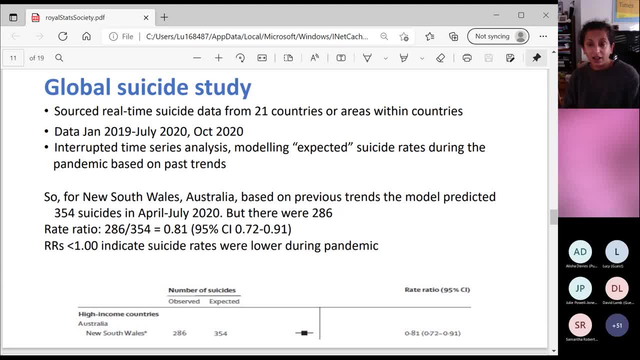 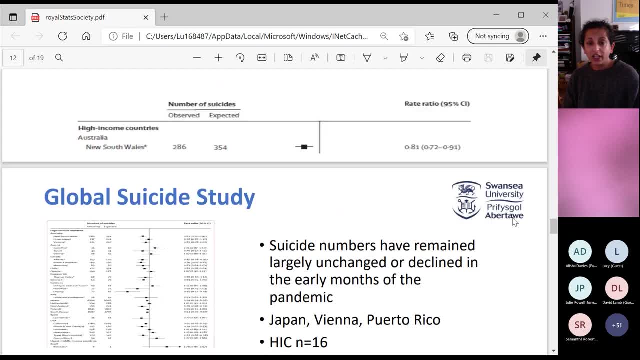 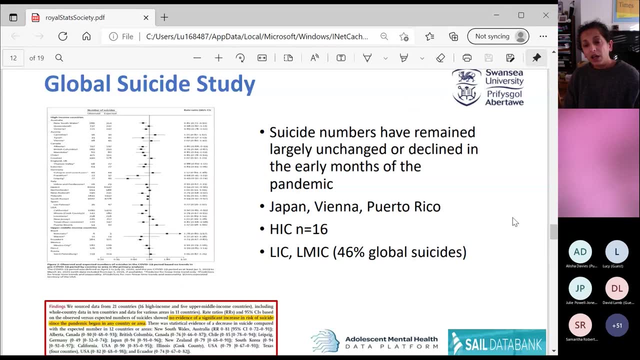 and expected uh data next slide and basically what we found was that suicide numbers had remained largely unchanged or declined in the early months of the pandemic. there were some exceptions to that, um uh, in japan it started increasing from october, but we think that was related to. 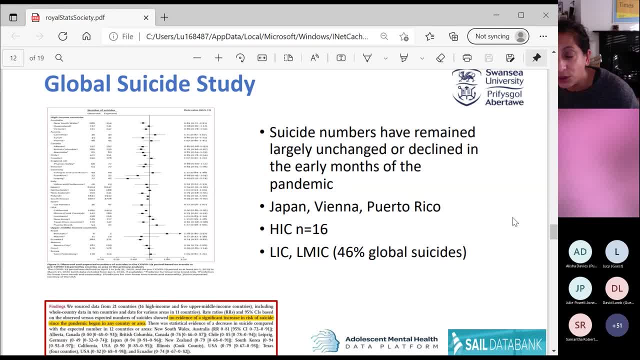 um, a celebrity suicide in vienna. we're not sure, uh, why it was different in puerto rico, and i think this was one of the beauty of this sort of collaboration. i think, in within statistics, it's really good to work with people who know the context and know the data, because when puerto rico 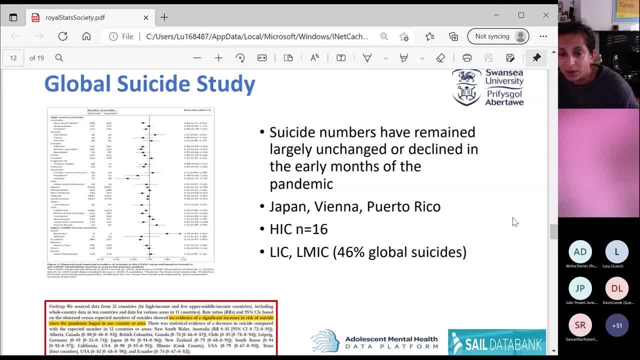 came up, we, we thought, oh, it must be about economic stresses, but if? but the people we were collaborating with specifically said that because of all the storms and hurricanes there people were still homeless, and so when covid came along, there was very little community with this, uh, resilience. 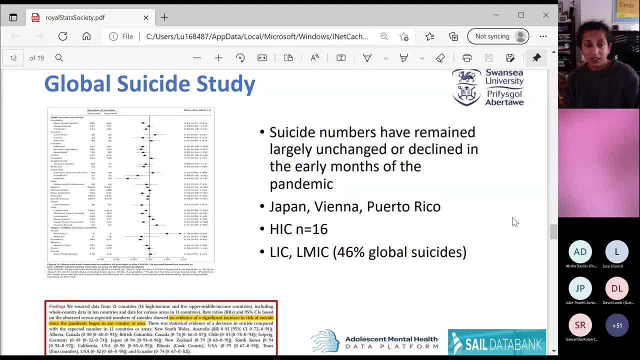 one of the weaknesses of this study- and we're redoing it so we've hopefully addressed it in some way- was um 16 of the 21 countries were high income countries and about 40. you know, over half of global suicides were in low and middle income countries and you know. 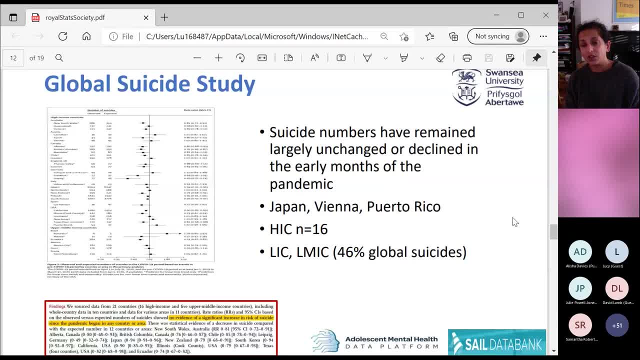 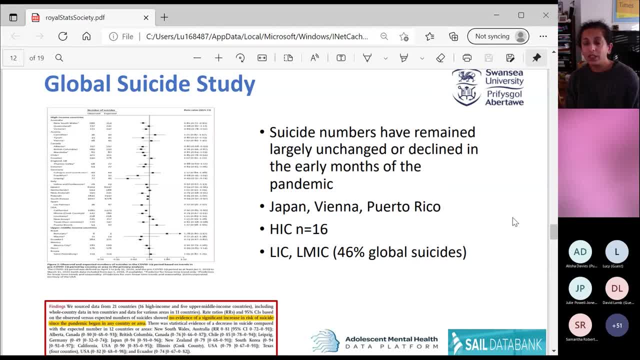 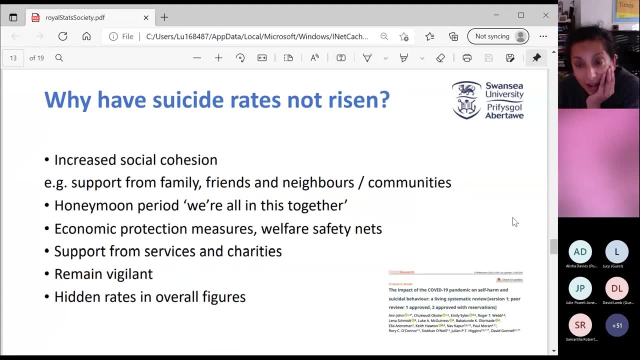 covert is happening to develop these sorts of information systems and i think i think that is a challenge for the sort of work that we do. next slide, next challenge was: you know, so people were so why hadn't they risen? so we, we think some of it's to do with increased social cohesion. 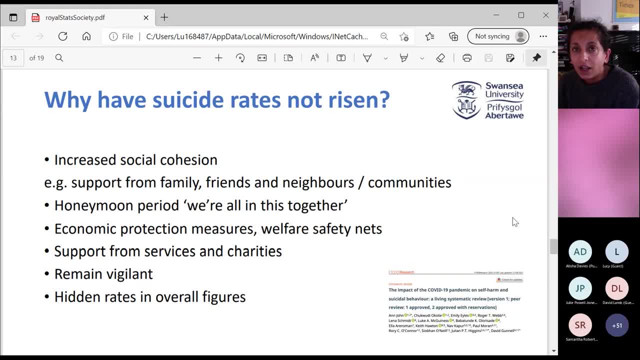 um you know, support from family and friends. lots of natural disasters are followed by this sort of we're all in it together honeymoon period. there were lots of economic suicide is strongly associated with unemployment and economic measures and, um you know, lots of things were put in place which, 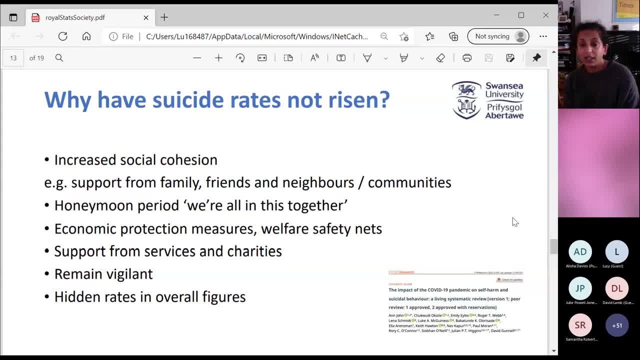 are disappearing now. um so we were constantly saying: remain vigilant. there was lots of support from services and charity and we're all in it together. honeymoon period: there were lots of things we were constantly saying: remain vigilant. there was lots of support from services and charity and we're all in it together. 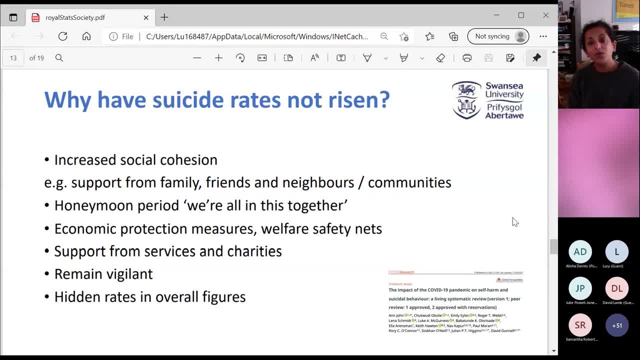 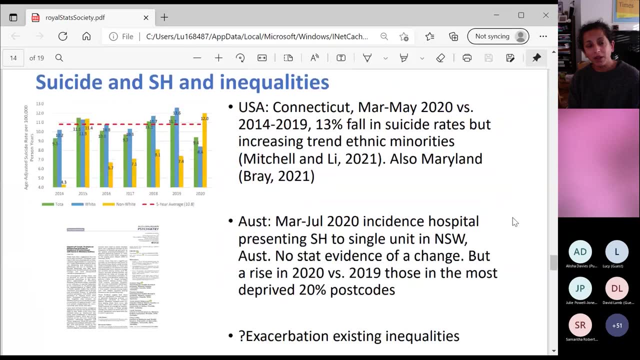 but- and i think this is one of the risks- so people were very reassured. um, there was an mp who actually said, oh well, we don't need to worry about that sort of thing, but um, next slide. i think it's always important that we remember that there can be hidden populations and trends within overall. rates, and so i think it's important that we remember that there can be hidden populations, and so i think it's important that we remember that there can be hidden populations and trends within overall rates, and so i think it's important that we remember that there can be hidden populations and trends within overall 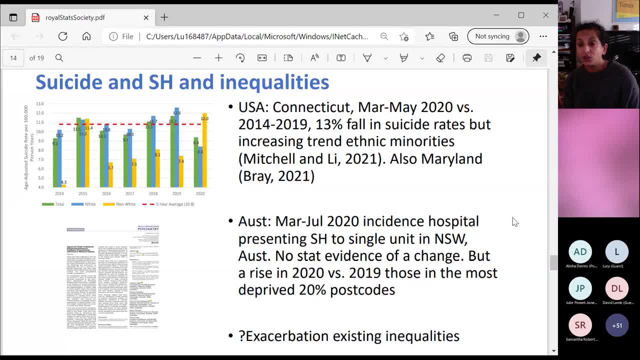 studies happening over and over. so there's a couple of studies that have come out of the states showing um: while there was a drop in suicide rates, there was an increasing trend in ethnic minorities. comes back to all that disproportionate impacts, inequality stuff and covered. and there was a study from australia about um deprived areas. so, uh, next slide. so we're. 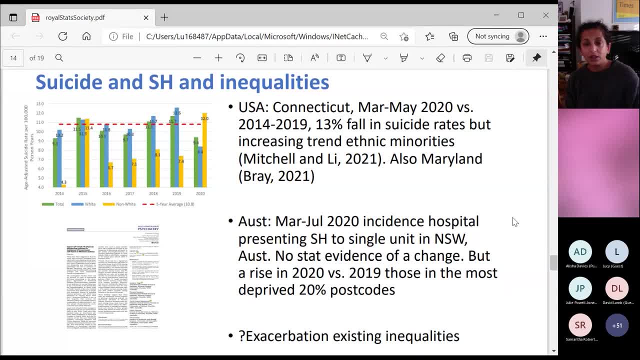 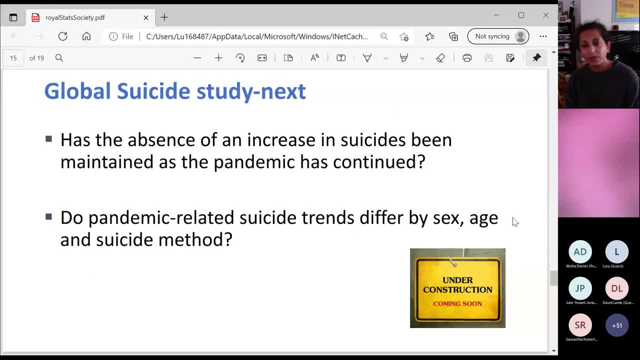 um deprived areas. so, uh, next slide. so we're, so we're, we've extended this exercise, we've got more up-to-date data, we're looking um differences by age and sex and at the moment I think we've got 48 countries, data from 48 countries. 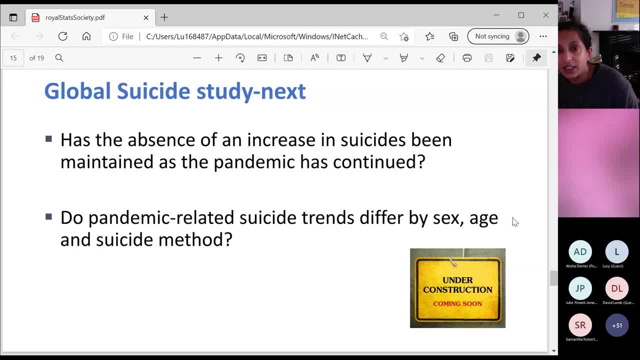 so it was one of the things I think COVID has done for our community. so people working with data is really foster collaboration, both across countries, jurisdictions and disciplines. you know, I've I've been working with behavioral scientists, sociologists, anthropologists, infectious disease modelers. it's, it's been really different. so what about mental health? 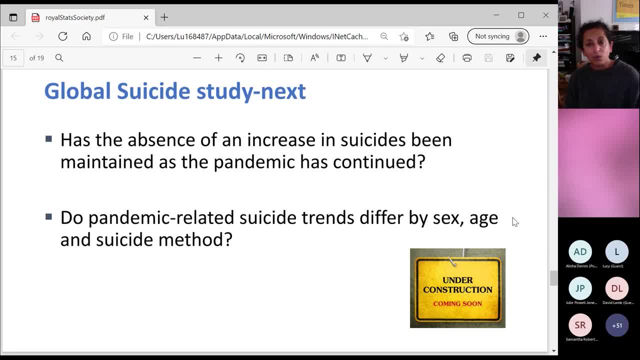 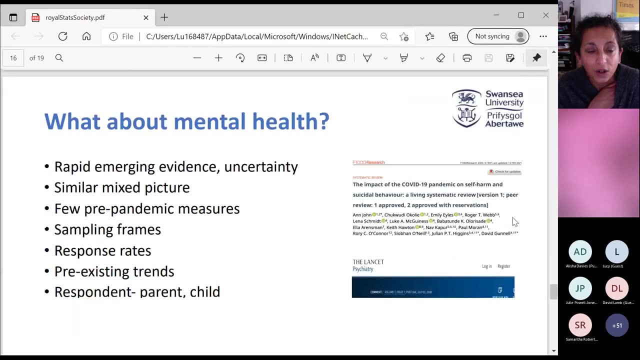 so what? what's been highlighted, I think, during COVID is when you've got rapid emerging evidence and we set up a living systematic review. so next slide is quality of life, quality of data. so you know, we saw loads of studies being published with no pre-pandemic. 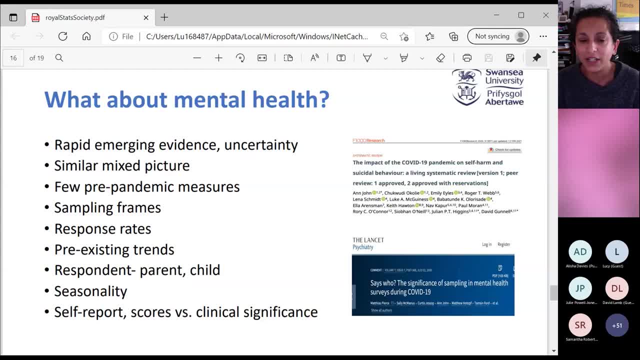 measures. so there was no concept of any pre-existing underlying trends. lots early on there was no discussion about seasonality sampling frames. the number of convenient samples that were, you know, splashed across the headlines without any of the caveats around that. when you're doing that sort of analysis, 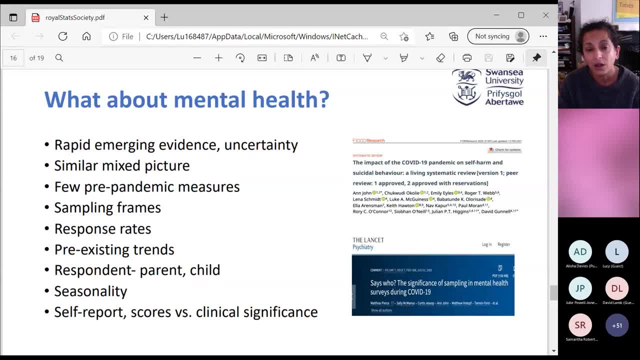 people literally ignored response rates. and then we talked about self-report on clinical significance. so I think it's really important that I mean- and I know you all know this- about the design of data. so even panel surveys, you know, don't measure the people who aren't in them, even though we call them. 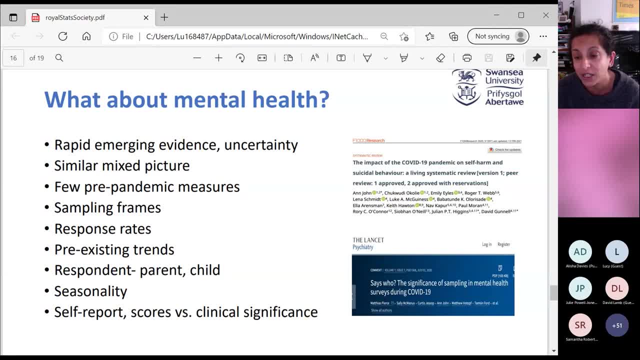 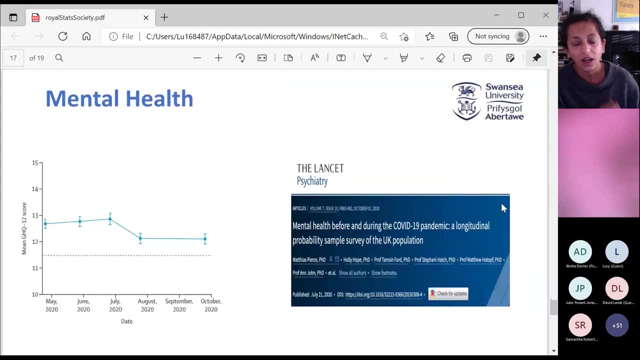 representative. so we wrote an editorial about that. called says who and we wrote an editorial about that about the significance of sampling in mental health. so I've got a couple of minutes. I'll run through quickly about mental health. next slide. so this is about GHQ. with GHQ, the lower the score. 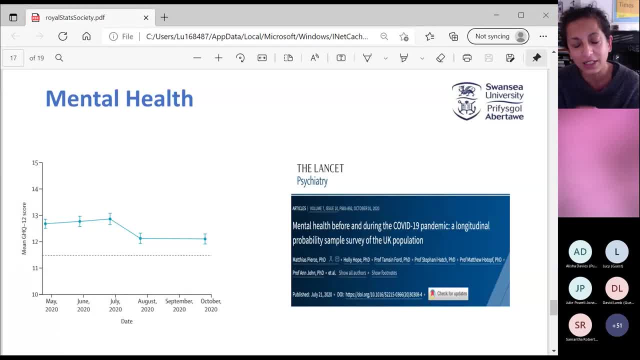 the lower the levels of mental health and it is. it does measure diagnosable mental disorders. so during the pandemic there was that initial drop which is the line going up in in mental health across the population. things improved a bit from July but we have not and continue not to have reached pre-pandemic levels. so 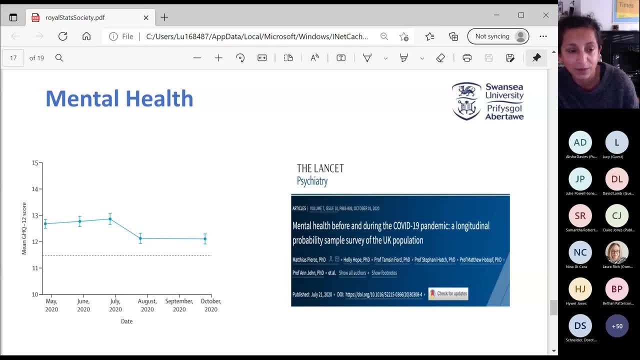 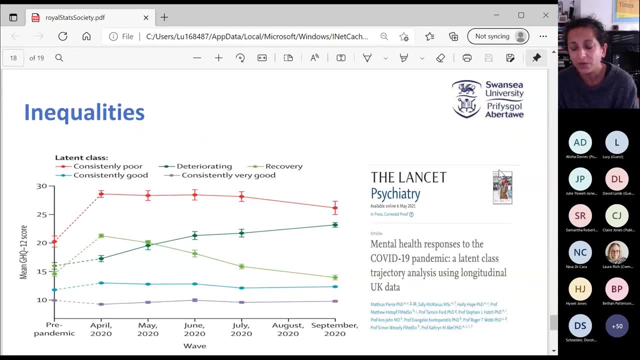 and then the next slide. um was a piece of work that I was proud to be involved with. it was led by Matthias Pierce in in Manchester and it basically we're using the understanding society um survey here, which is a probability sampled um cohort, and we basically did a latent class analysis and what we identified was for about 70 percent of the population, so the 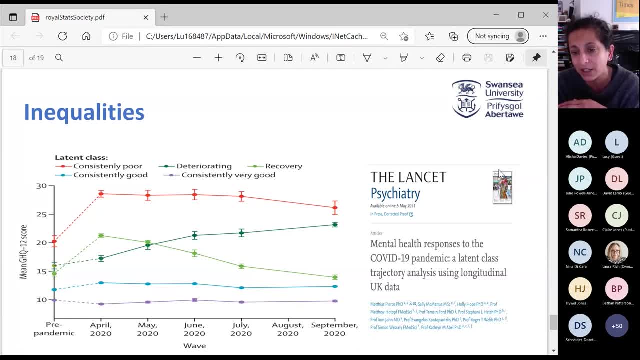 light blue line and the purple. they were sort of consistently okay during the pandemic. the light green line showed people whose, whose mental health sort of deteriorated immediately, you know back in march, april, but then they sort of recovered as well. and then we're left with the 11 percent of. 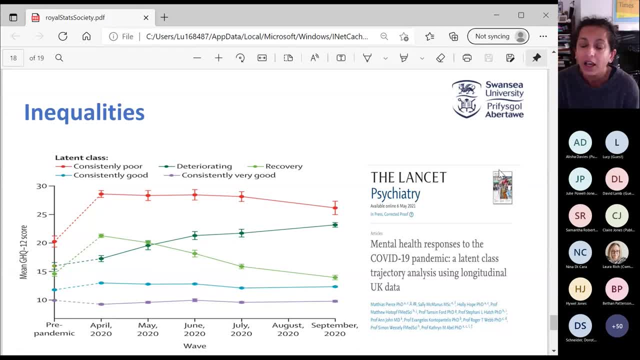 the population with the red and dark green lines and with those people. their mental health was either consistently poor throughout or deteriorated, and within those two um. those two groups were young people, people from ethnic minorities, people with pre-existing mental and physical health problems and those from deprived communities in terms of um, employment and 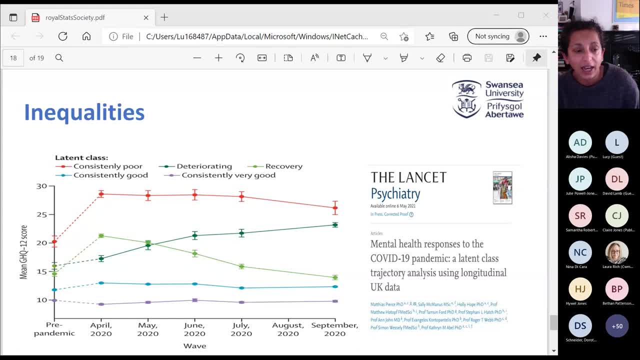 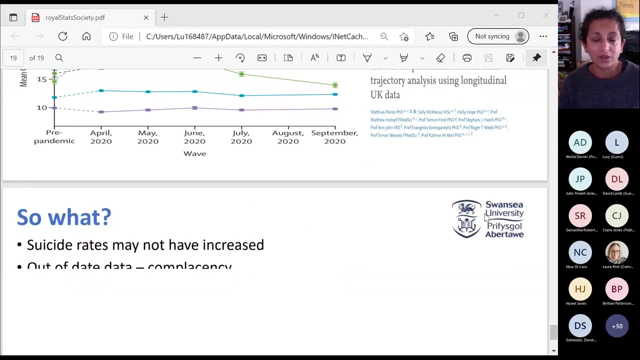 an income. so i think it really highlights how, um i guess, the disproportionate impacts of of the pandemic and i and i'm really do think people working in epidemiology and statistics have really been able to put evidence behind what we all know to be true um next slide. so what's the point of it? all you know? 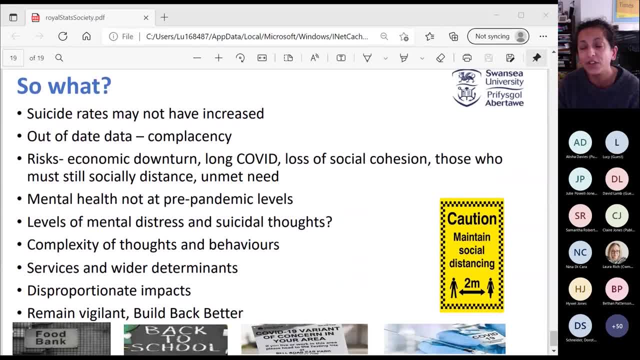 i think we always have to. one of the challenges of everything that we do is that so much of our data is out of date by the time we get it out there. i think you know it used to take 18 years to get research into practice. i think covid has shown us that that doesn't have to be the case. 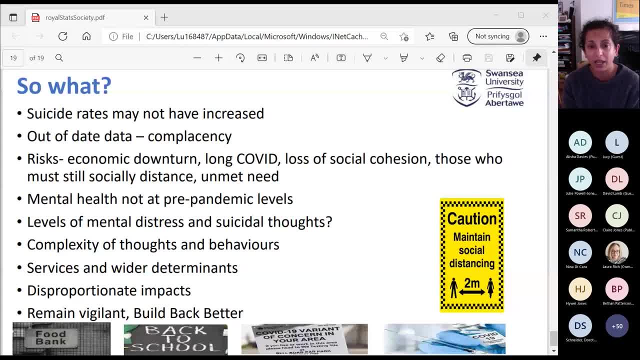 um, i really don't want to go. go back to that place. that the risk going forward, you know economic protection is going economic downturn, that loss of that social cohesion impacts of long covid. um and all the unmet need of people who didn't contact services. mental health still isn't. 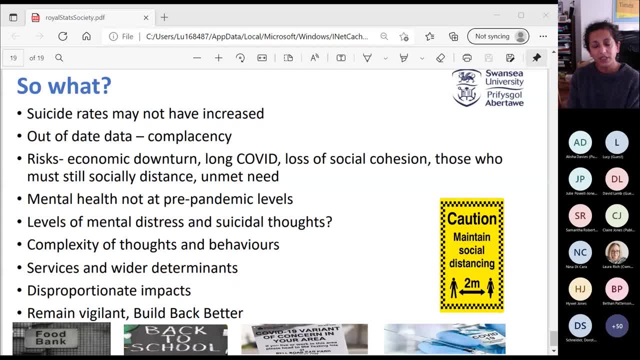 at pre-pandemic levels, you'll see a lot of people who didn't contact services who didn't contact services. so there's a lot of stuff out there about increases in suicidal thoughts and um it. it does look like that did happen, but there's a very complex relationship between suicidal thoughts. 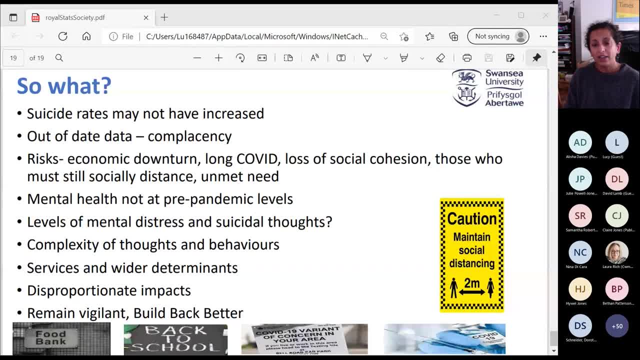 um, progressing to behaviors, and i think that sometimes you know, i think when we report on things, we have a responsibility to talk about those, those issues, um. so i guess my two big messages is that you know, i think it's a very complex relationship between suicidal thoughts and 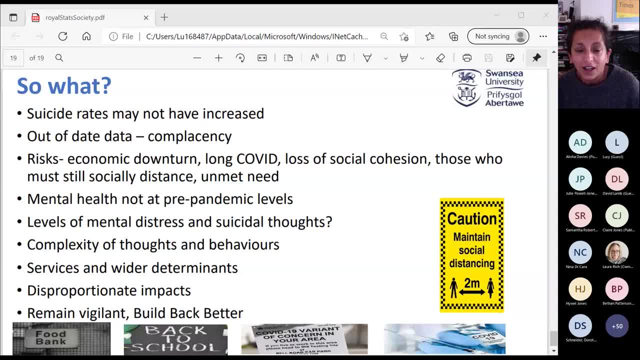 you know we all have to. i, i guess as a society we need to remain vigilant, and part our role in that is is to keep providing the evidence about what's happened and who it's happened to. and you know, i just put bills back better because i hope we do, but the last two days makes me slightly um unhopeful. thank you. 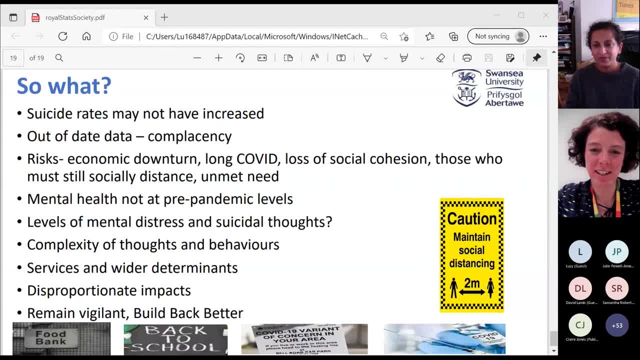 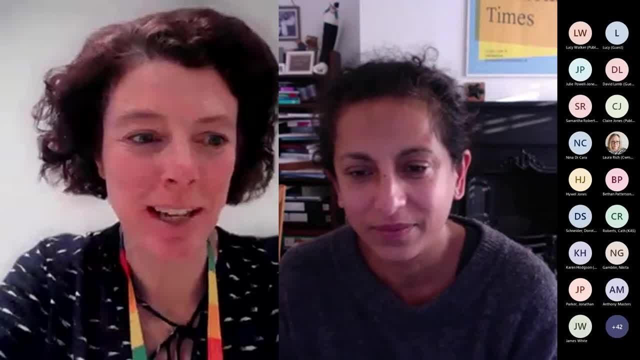 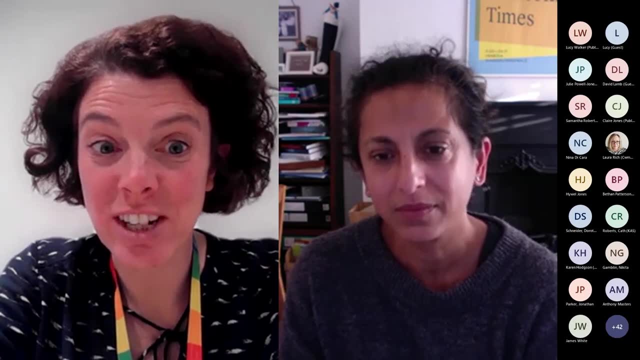 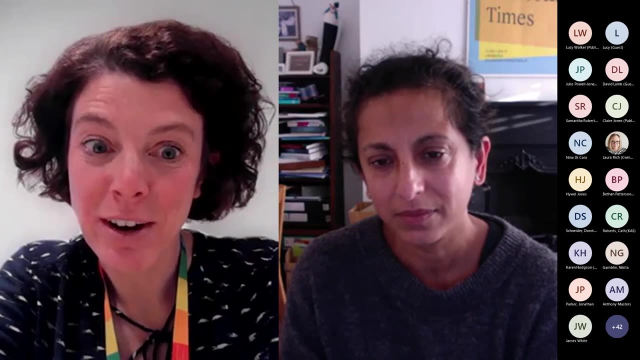 thanks, anne. um, that was just fantastic. um really fitted with the title of today. so kind of challenges, challenging statistics in public health, both in the generation of those statistics and also the challenges in the messages that the data shows. actually, um and and really highlighting some of the disparities, both in the direct and the indirect impact of of covid. um, i'm fascinating. 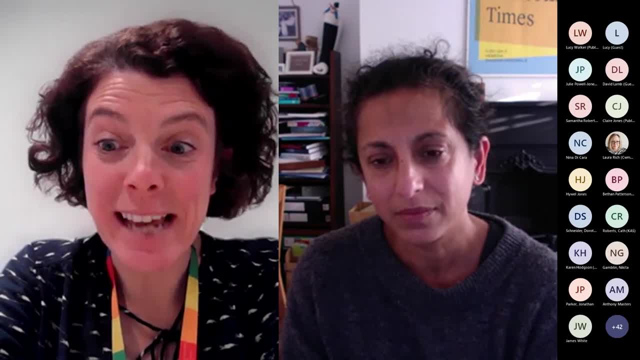 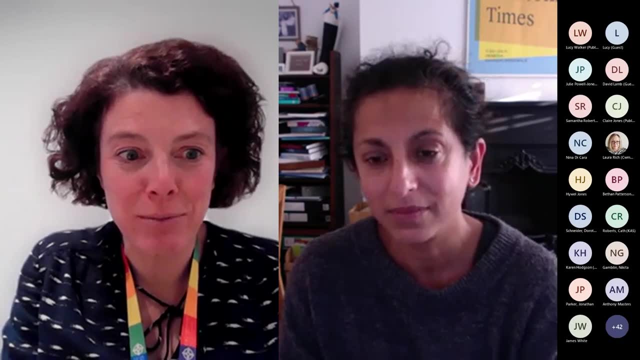 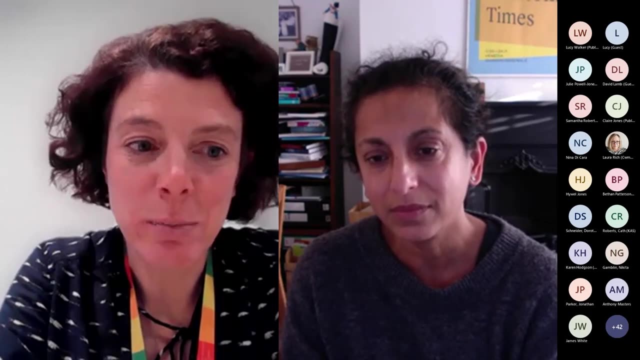 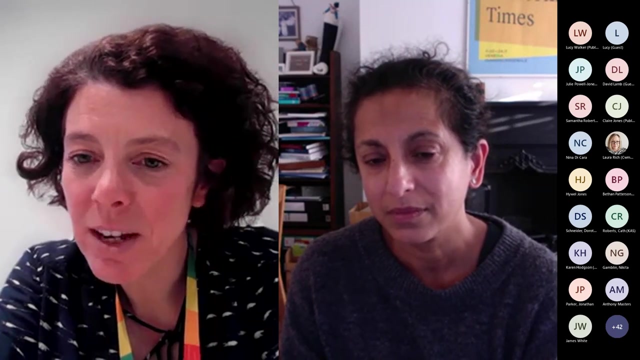 to see how this, how it took a pandemic actually to get the international collaboration, the use of the tre or the trusted research environments, that kind of speed, that um, sometimes, um, academia doesn't tend to move at that speed, but you know, it's certainly demonstrated that it can. um questions from the. 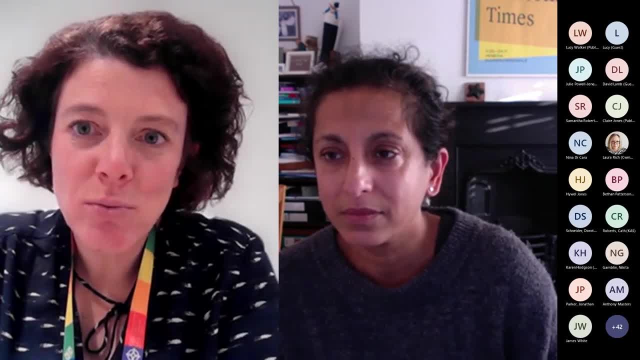 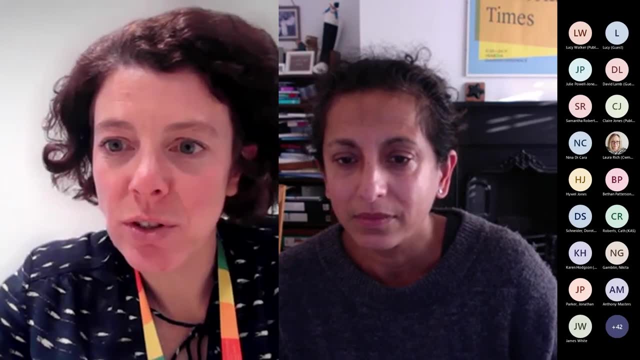 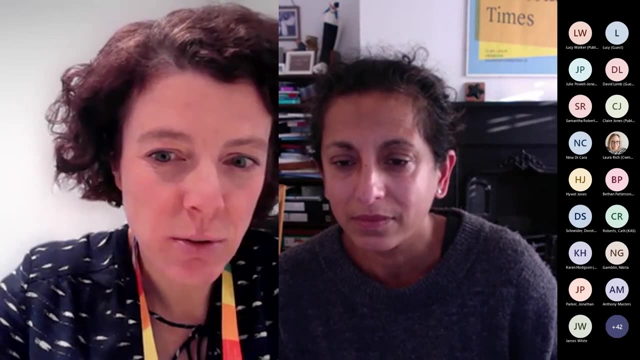 audience or anyone wants to um, ask a question for ann. do pop them in and um, or pop your hand up, um, and if, if you, if you do, then just um shout and really handy as well. and is it okay for us to share your slides? i should have asked actually before, with the group later, yeah, yeah, yeah, later, maybe. 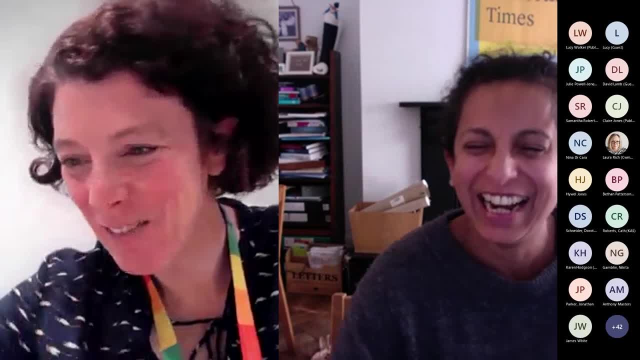 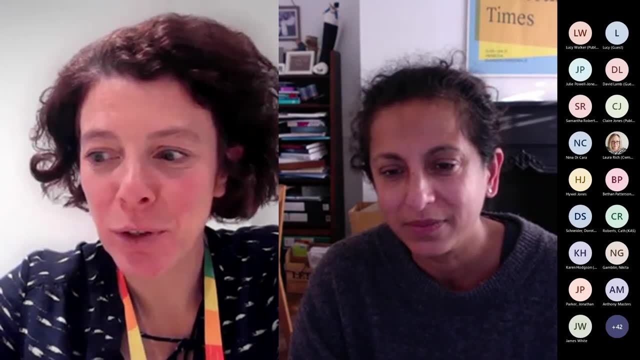 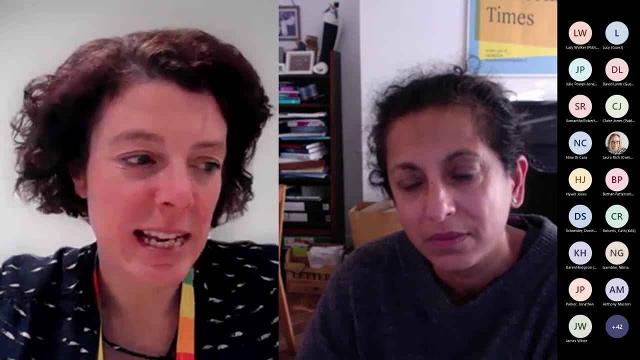 tomorrow would be better post publication. fantastic at the paper eye. um, wonderful um with um. i've one question for you, which was um a really interesting one. that was kind of a one that you popped in at the end about um, the ability in linked data to um identify people. 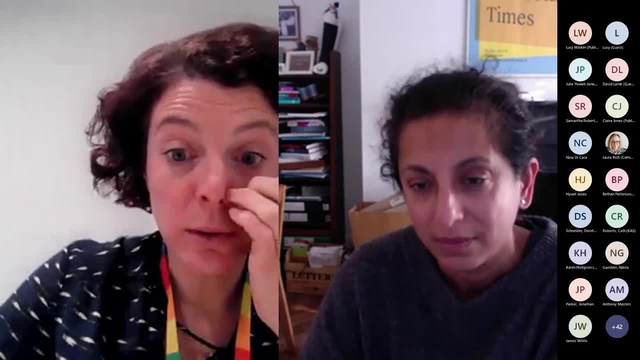 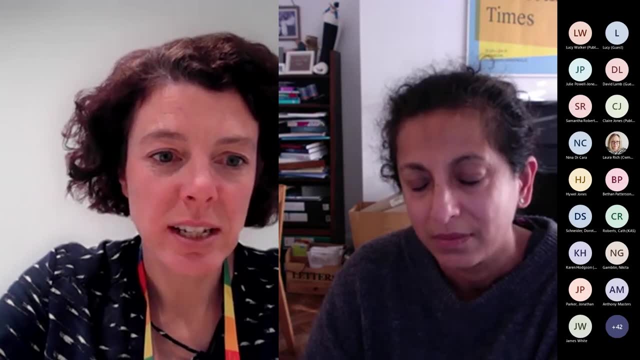 early that might be in need of more support in that school environment in particular. there's a lot, isn't there, on whole school approaches to mental health, um, and supporting individuals. i'm just interested is there, is there something in the wings that's developing in that space? 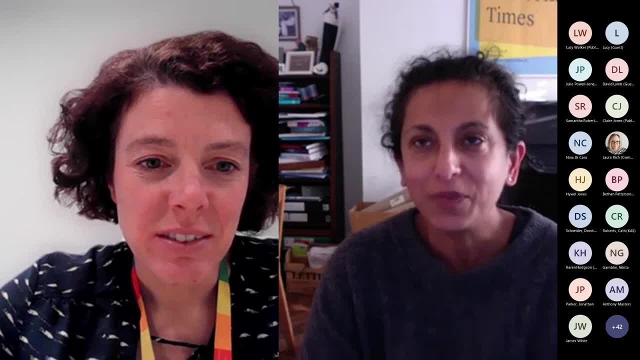 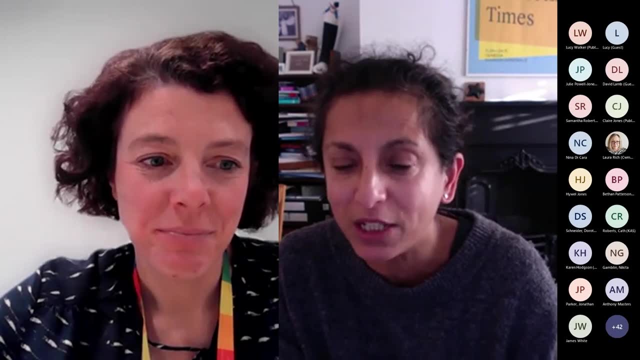 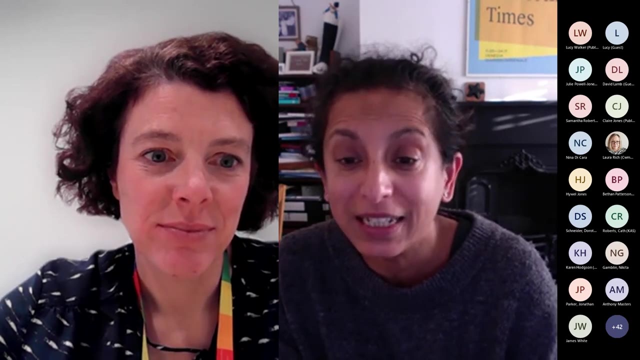 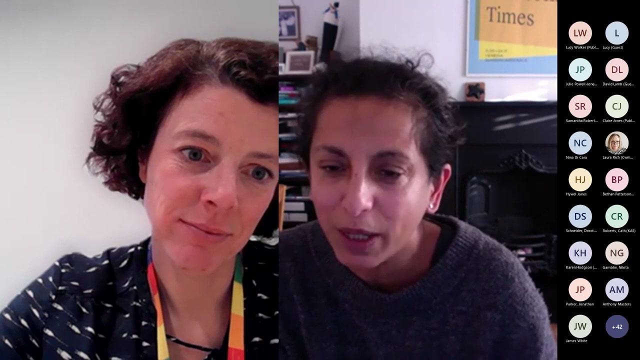 um, i, um, so there's lots that they they've set up already. I think over the last few years there's been a real transformation in that recognition of schools as a place where we can deliver and support. but I think we're hoping to use this and some of the other papers we've done in in this area. 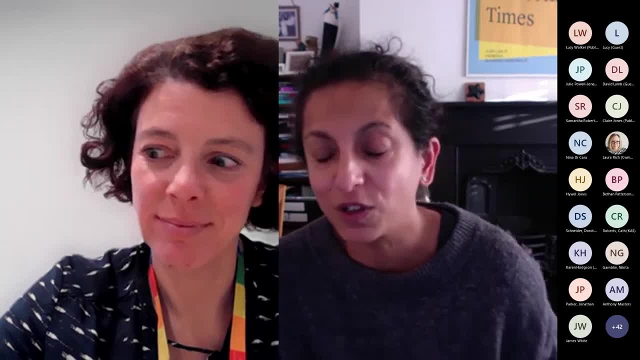 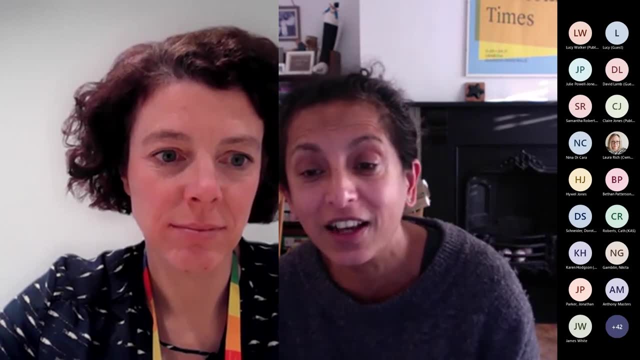 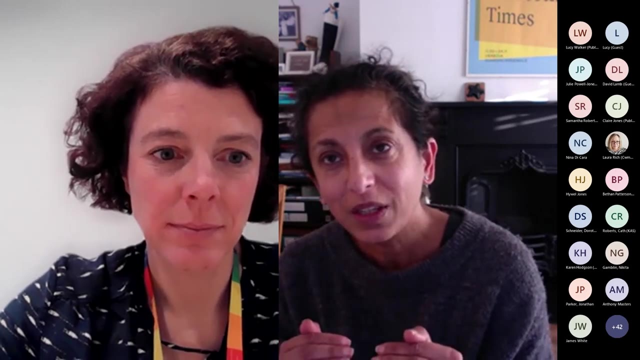 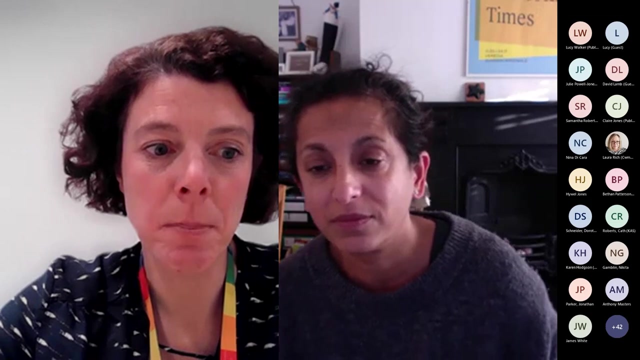 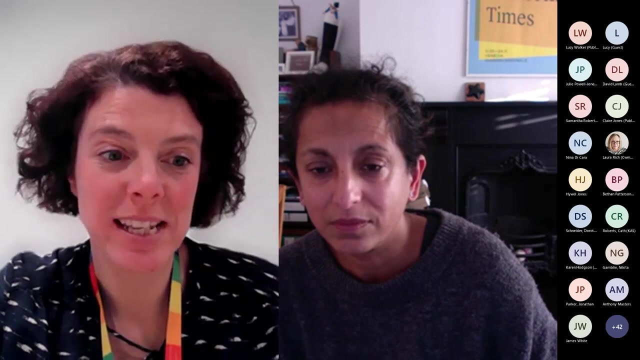 to to work with others across the country really to make more use one of the data that schools generate, because really they can identify these young people themselves and then use that to push for more integration across education and health. Fantastic and that that generating that evidence, much as was done there with the suicide to inform the policy action in that in that space. so how can? 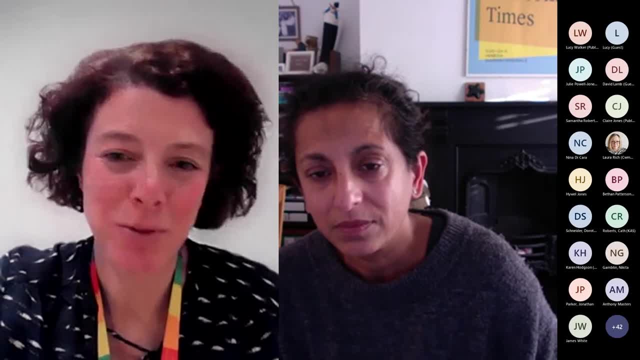 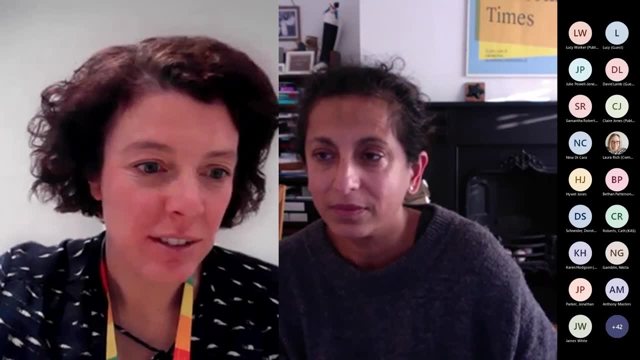 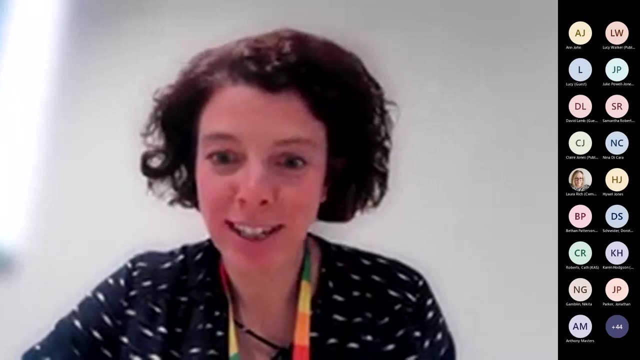 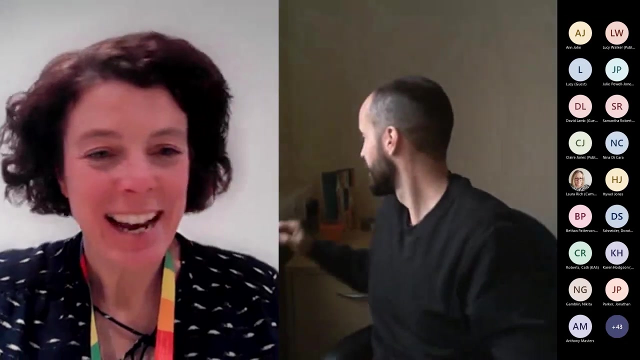 we get more up, but well, upstream, downstream and the prevention, Fantastic. thank you ever so much and we'll. we're moving on now to our second speaker this afternoon. just need to remind myself of our running order. James- I hope James is there somewhere. James White from Cardiff University, you are. thanks, Jim, and welcome. welcome. thank you for joining us this. 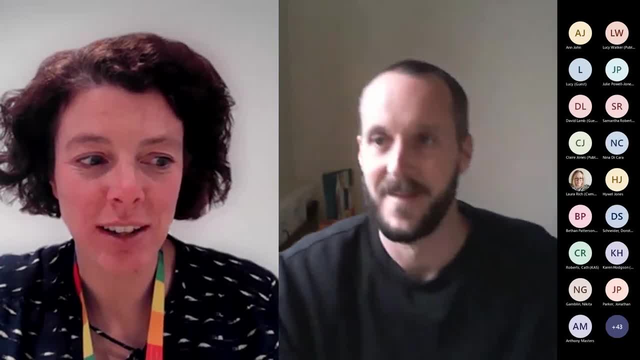 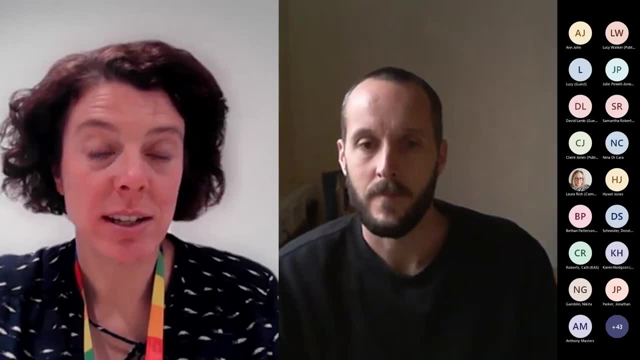 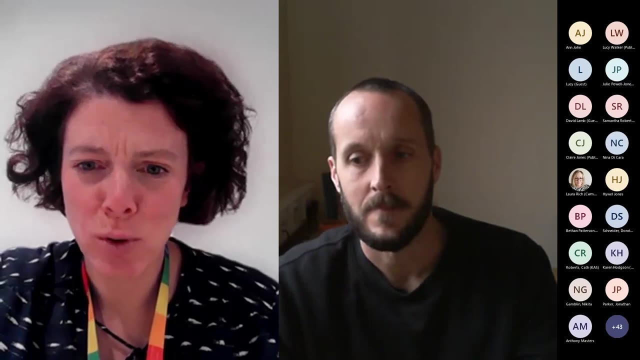 afternoon. James is a deputy director of population health trials in the Center for trials research here at Cardiff University. Thank you, Thank you. I'm James White from Cardiff University in Cardiff in in Wales, and based in decipher, which is the center for the development, evaluation of complexity and implementation in public health. 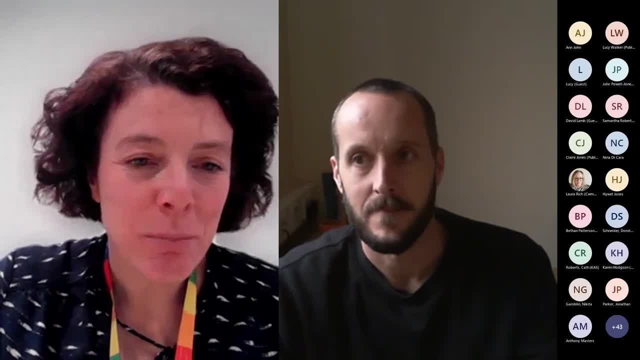 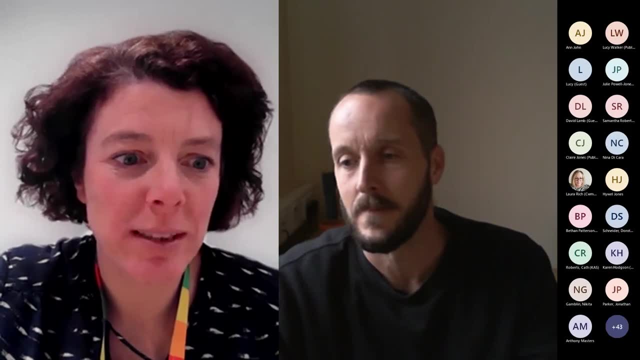 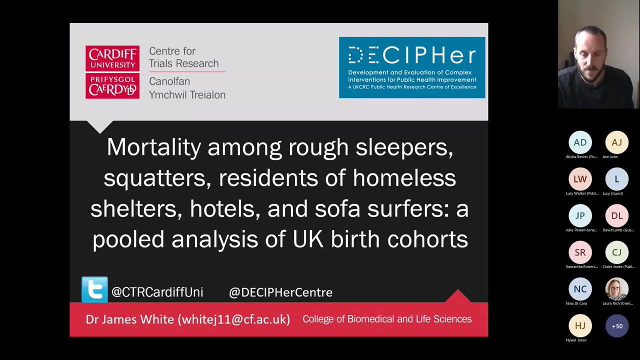 rules off the tongue and so James over to you and yeah, any questions and things, feel free to put them in the chat as James is talking and we'll pick them up at the end. James Anne's team yet quite nicely in that, a lot of the focus of her work and some of the drivers that 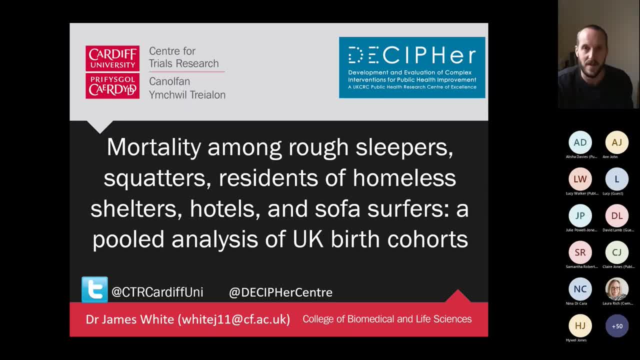 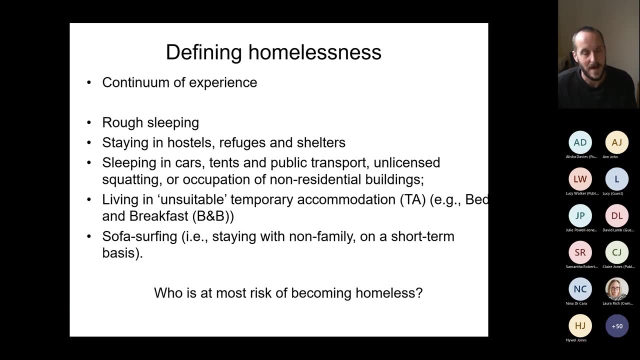 have met. our problems are experience of socio economic disadvantage, inequality. I want to talk today about one of the more severe and extreme forms of disadvantage, namely homelessness. so Just to talk a little bit about definitions of homeless, many of you will senior daily lives people roughly think, and some of you may well, in your cities and towns, be aware of homelessness and 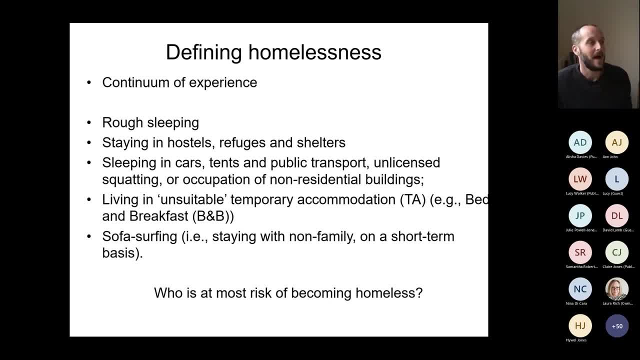 hostels and refuges and shelters, um and these are the most visible forms of homelessness and um form. the majority of research into homelessness has been on rough sleeping and hostel people who stay in hostels. but there is other forms of homelessness that also exist. for example, i put there sleeping in cars, people squatting, and there's a a larger group of 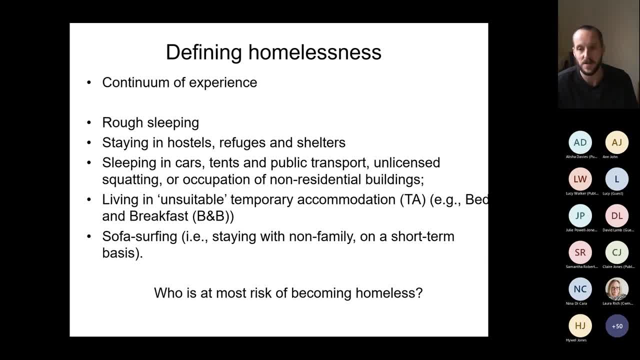 individuals who, for example, live in temporary accommodation such as bed and breakfast. these may be single occupancy rooms with shared bathrooms and shared kitchens, and also sofa surfing is a form of homelessness where most people first land when they become homeless. just to contextualize homelessness a little bit, although it might be useful just describing the 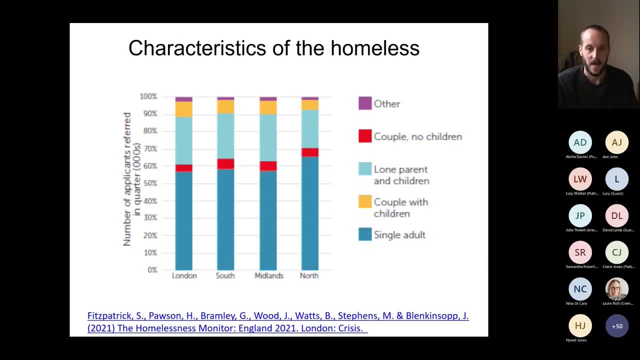 types of individuals who are most risk of becoming homeless. so this is a slide from a annual report. this is the 2021 report from susan fitzpatrick. that is sponsored by crisis, and what this shows is this is data from people who present in local authorities. 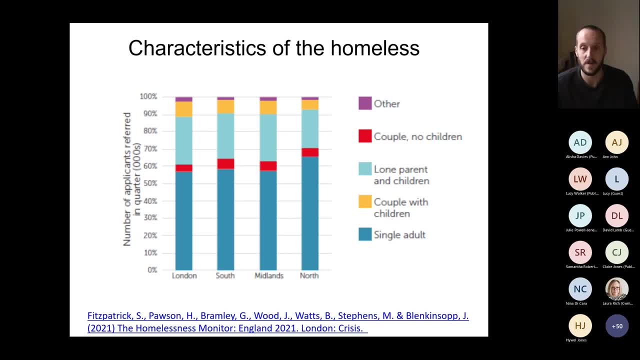 for help with their homelessness. they're at risk of becoming homeless. what it shows is that the majority of people who present are single adults, in particular single adult males, and then the next largest group is lone parents with children. another groups are less prevalent. this is a study looking at data from the british birth cohort study. 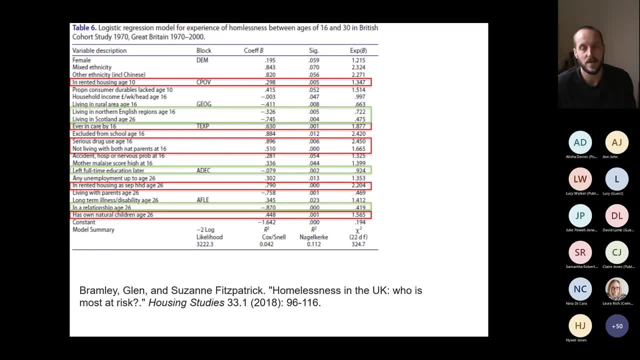 this is data which is looking at exposures recorded before the age of 30 and trying to predict the individual's risk of becoming homeless by age 30 and later on. i'm going to be presenting some data from the british birth cohort study, so this provides some useful information, and so i've 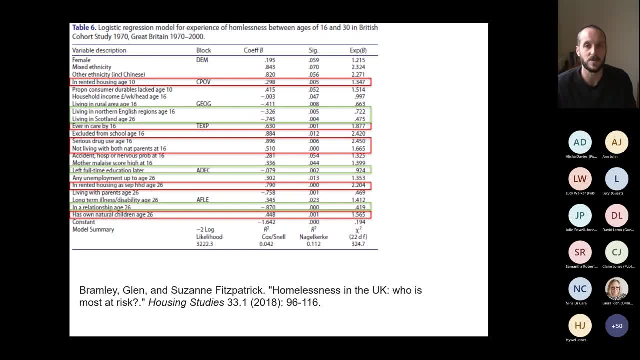 ringed in red there the uh factors, which are associated with an increased risk of becoming homelessness, and then mainly people living in um rented accommodation, people who've been care experienced, use serious drugs, not living with natural parents, um, and also living in renting housing later on in their early adult life as well. and across the data and across a number of 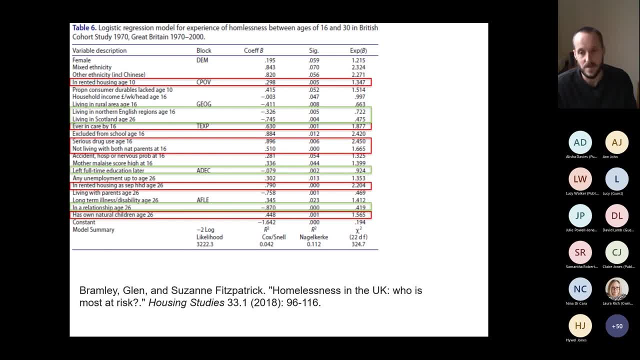 studies um, what you will find is that individuals who are at risk of homelessness, uh, are much more likely to have a childhood that is characterized by socioeconomic into disadvantage, unstable housing. they're often care experienced, report mental health problems and have lower levels of educational attainment. and i've just written some green factors there which are 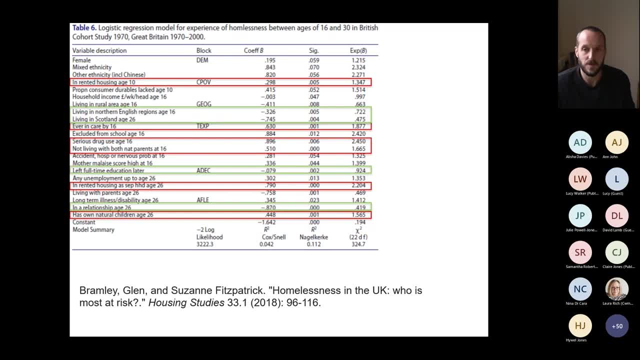 factors which reduce the risk of an individual, or associated with a reduced risk, of becoming homeless, and some of these are geographic. so people living in northern england and scotland were less likely and this is likely to do with the availability of social housing stock and different levels of deprivation across. 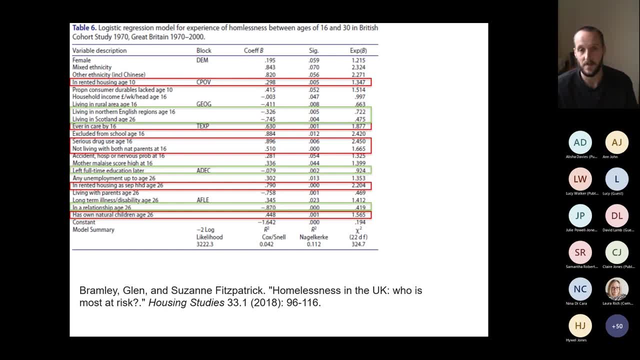 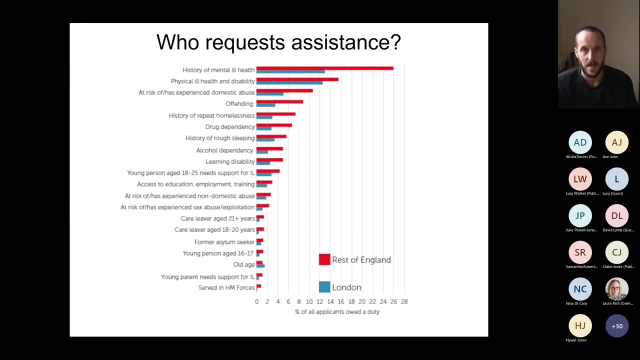 devolved nations. they're more likely to have left full-time education later on in life and also being in relationships. so that may be because people in relationships- um, you have two business. they provide a bit of financial ballast to unemployment. this is data from people who report in local authorities for for assistance and this kind. 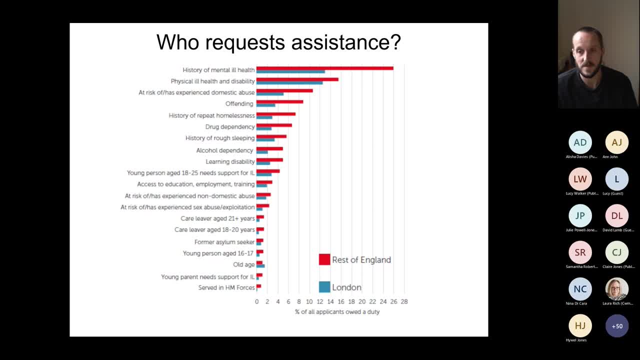 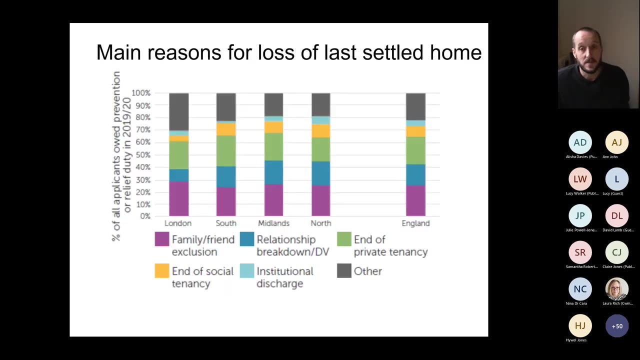 of chimes. with the cohort data, the people who report for assistance for homelessness are much more likely to have a history of mental health problems, physical health problems, experience domestic abuse and you can see some other risk factors there. this is the reasons when people report for health. they're asked about why they become homeless and it's a real mix of reasons. 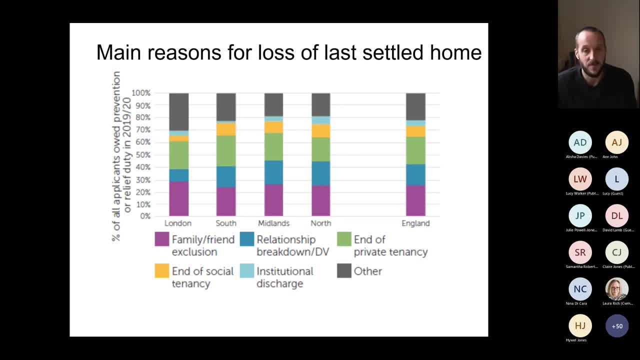 that kind of aligns with some of the risk factors. so family and friend exclusion, people being left are to leave home. young people being left less delete, asked to leave home by their parents. um breakdown relationships and domestic violence, ending the private tendencies as well. moving on now a bit to show a bit about um prevalence. 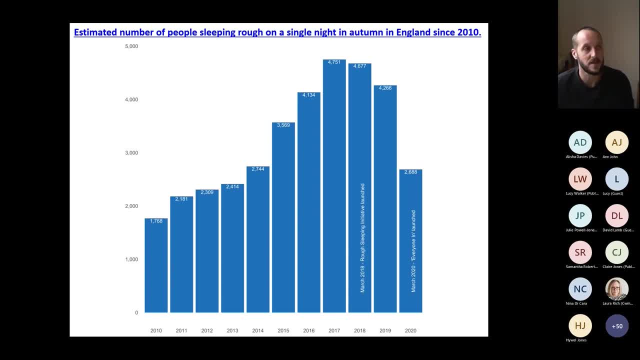 so this is data from a annual survey that's conducted every year, where they count the number of people rough sleeping, and what it shows is that between 2010 and 2017, there was a large increase in the number of people who were rough sleeping, um, and then in 2018 it kind of 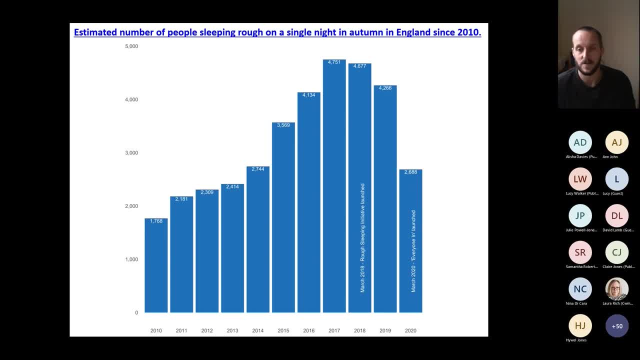 leveled off with the policy initiative to target and reduce the number of people rough sleeping, and then a sharp decrease was found in 2020, and that coincided with something called uh the everyone in initiative. that was when, um, in the first wave of the pandemic, people who were rough 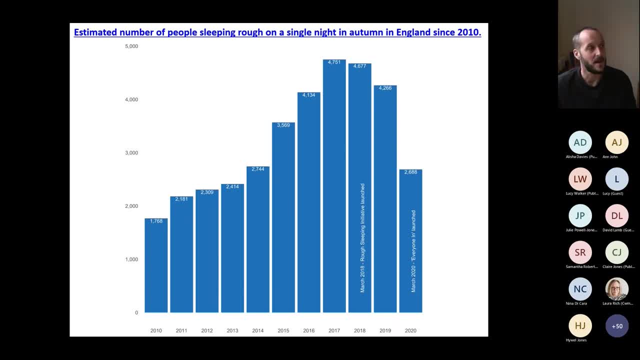 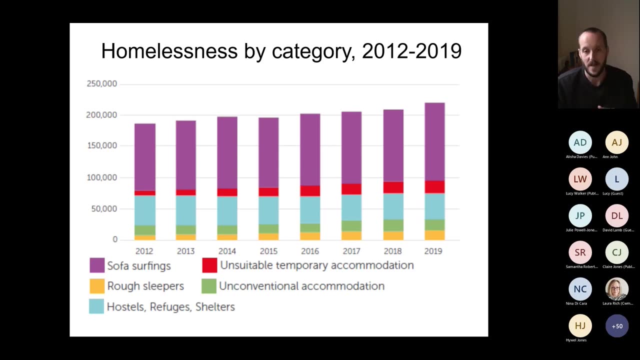 sleeping and also people in homeless shelters. uh were given access to hotels to reduce the risk of transmission and that was probably mainly in terms of the hostels. that's mainly because people sleep in large communal areas. in terms of category um, if we look at this is um homelessness by category. 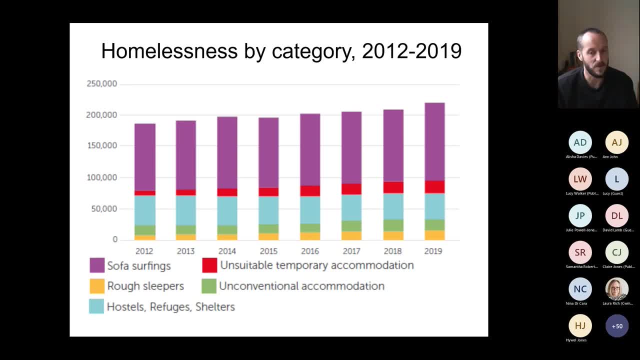 over time, and although rust, sleeping is more the most extreme forms of homelessness, it's by far the most the smallest proportion of homelessness across time. that's the yellow bars across the bottom. um much larger groups are people who live in hostels and the largest group by far are people who um. 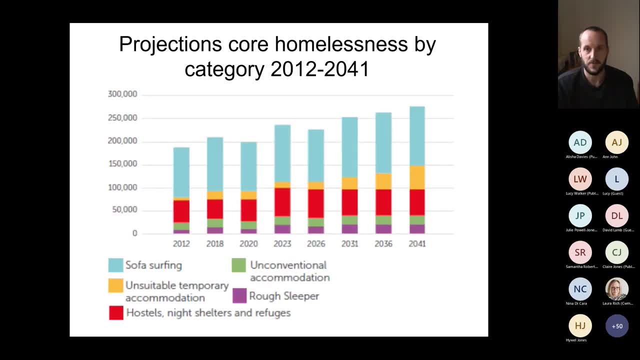 sofa surfing. this is a prediction from the crisis report um on trends of homelessness categories and that, whilst you know, sofa serving remains the largest group and uh rust sleeping the smallest group, one trend i would note is the yellow bar there, which is the use of unsuitable temporary accommodation. uh, and this is being occurring in more and more. 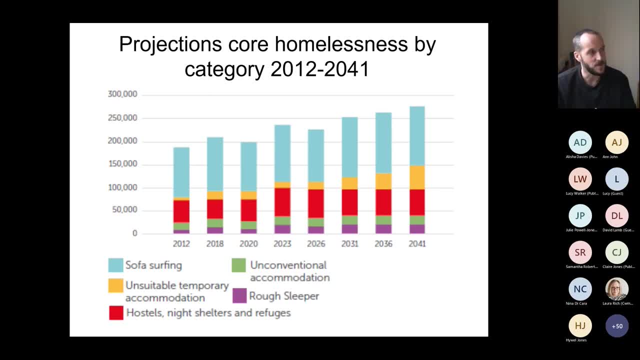 frequently in recent years. um and in part is due to uh increases in the pricing of uh rents in the private sector, lack of availability of social housing stock and it's likely to also be exacerbated by uh post brexit and covert related inflationary rises and costs. if we look at 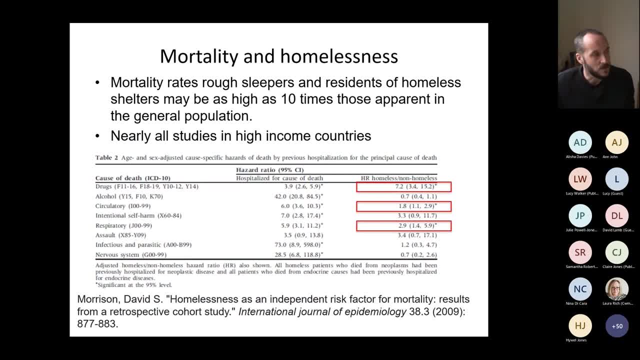 mortality in the previous literature. um, so the evidence here can be quite stark. so the mortality rates in some studies that uh look at people who are currently rough sleeping or staying homeless and shelters can be as much as high as standardized utilities, can be as much as 10 times that, as in 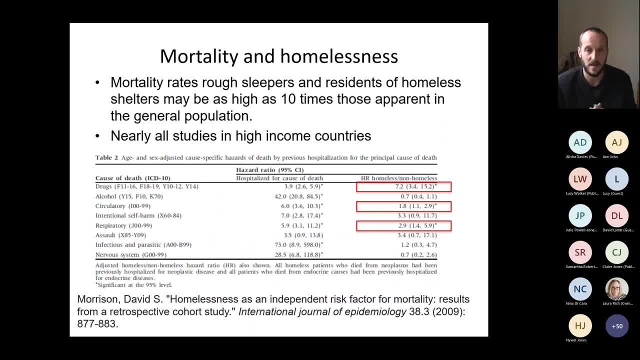 the general population. nearly all the studies are conducted in high-income countries. i've picked out this table from one study which is a record-linked study in scotland, and it kind of exemplifies what findings from others, which is that we see um particularly high rates of causes of death related to drug use. uh higher rates of circulatory cause of death and respiratory causes of death in those who are people who uh in this study were uh homeless because they had a no fix the bone indicator on the mortality record in comparison to the wider population. 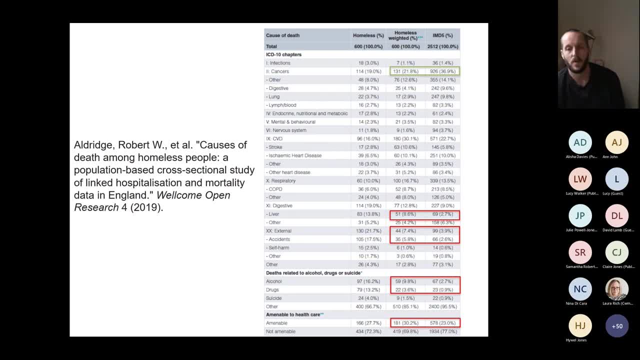 this study is by rob oldridge and colleagues in ucl and what it does is it does it? it kind of extends the previous study by having a comparative group- this is the far right column- who are people in the most deprived live in the most deprived quintile. 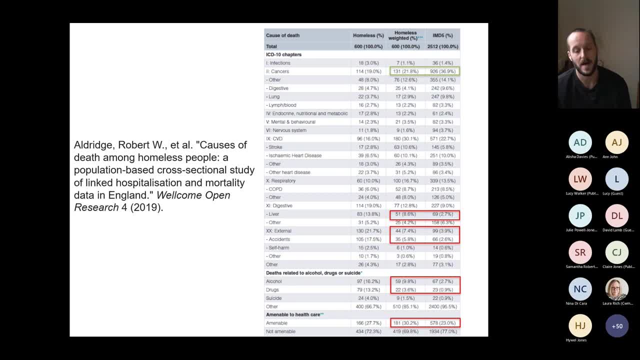 areas in england, and these are people who are asking for assistance at hospital and report that they were homeless, and what it shows is that, um, similar to this, the previous study, external causes of death, for example accidents, uh, others like liver disease and those attributed to drug. 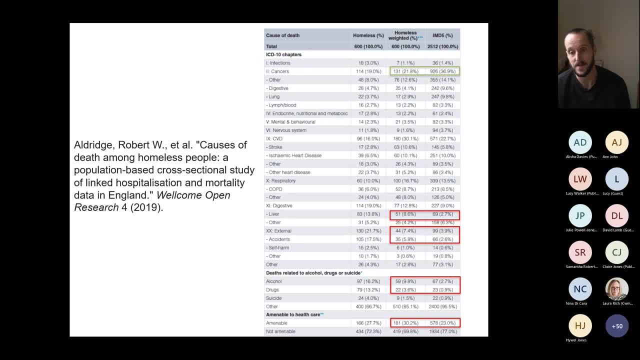 or alcohol use are much higher in the lower right column than those in the upper left column and so in the homelessness than the deprived comparison group. um, and i've also written in green there that, uh, the reverse was the case for cancers. so cancers were more prevalent in the in the deprived group. 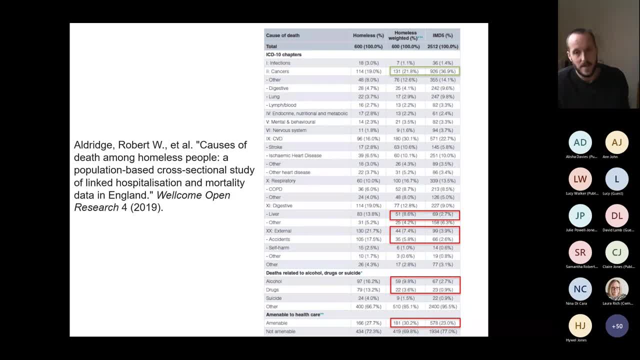 than the uh homelessness group, and this probably is due to the fact that it takes some time for numbers of cancers to accrue and that if people are dying at a younger age, for example from external causes, we're not seeing as many in the homelessness group there and that they calculated 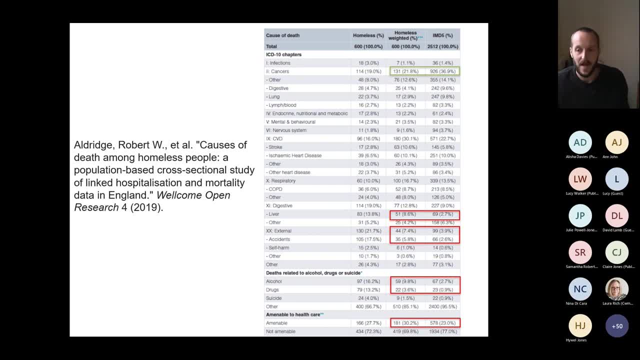 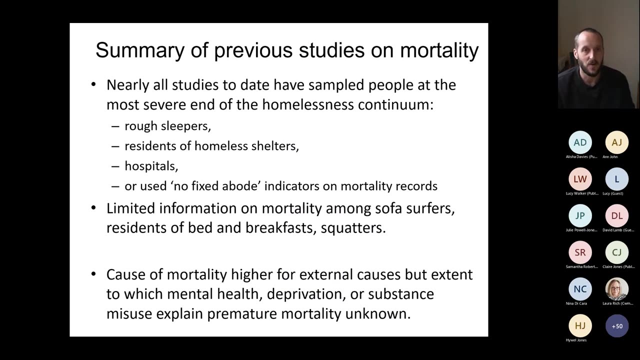 a proportion of these deaths were amenable to health care, and around a third of them in the homelessness group were deemed to be amenable to treatment, suggesting there's an unmet need here. so to kind of broadly summarize the previous studies on mortality- nearly all of the studies- 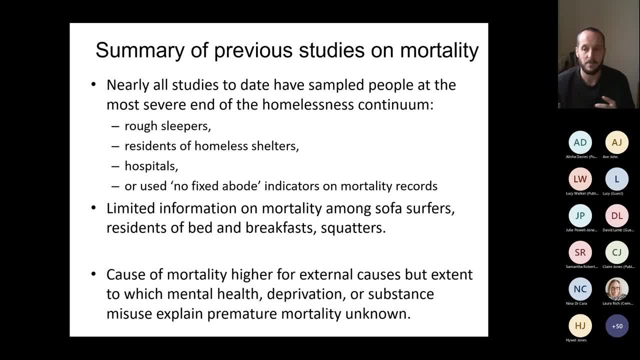 have cons of sample people who are currently homeless and are in the more uh severe end of the homestead continuum, namely rough sleepers and those in homelessness shelters, as well as other things such as uh using the no fix the boat indicator. there's very limited information and almost no studies. 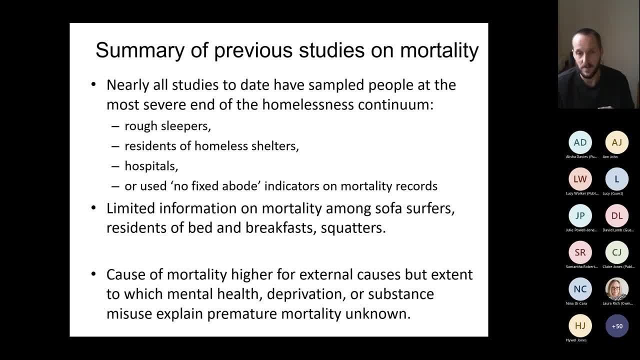 on the much larger group of people who are sofa surfing, those people who live in bed and breakfast, and then another group, which is a not large group but it's been admitted, which is people who squat. there are some notable differences in terms of cause of death and prevalence of cause of death. 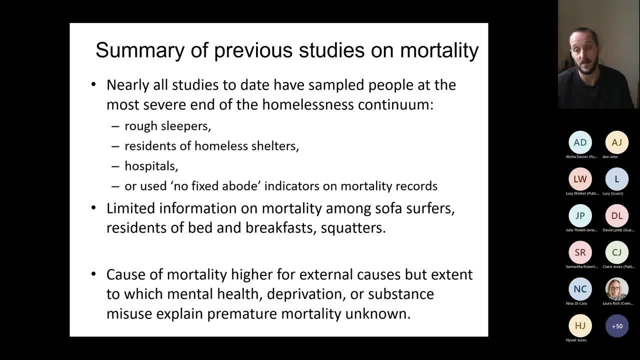 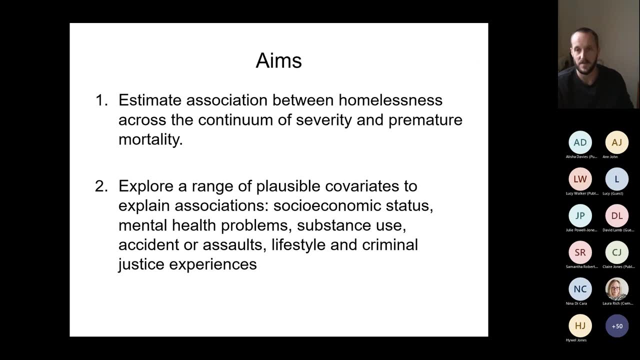 rates, external causes and other factors which are higher in the homeless experience than others, but very little information on the other factors that may explain these uh differences. so the overall aims of the study were to look at, estimate the association between homelessness across the full continuous severity and 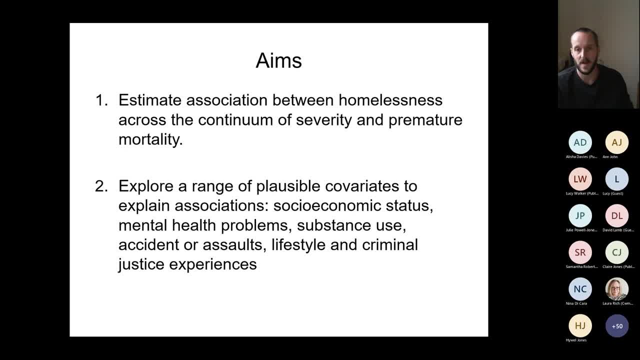 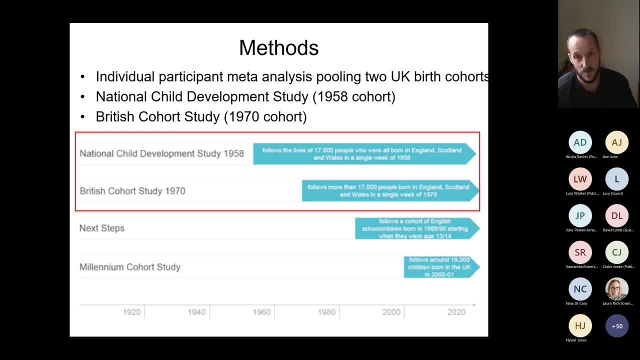 premature mortality and explain a range of plausible covariates to explain associations, and i've listed a few there. so, um, we use data from two birth cohorts. so uh we uh conducted analysis in each birth cohort and then we pooled them in an individual participant analysis. the two birth cohorts we use with the national child development study and the british 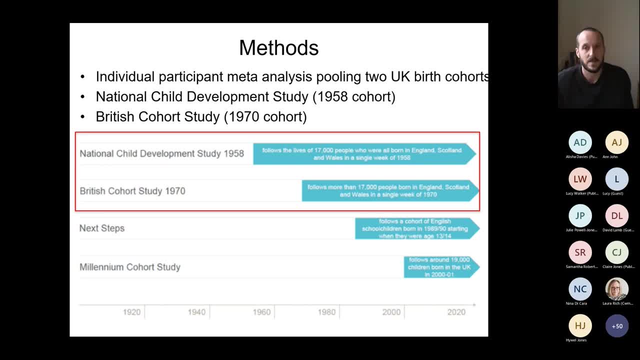 birth cohort and uh, i'll be calling these 1958 and the 1970 cohort because that's when they started. and uh, these are ongoing birth cohort studies that, um, sampled individuals were all born in a week in 1958 or 1970.. um, some of the good things about these birth cohorts are the 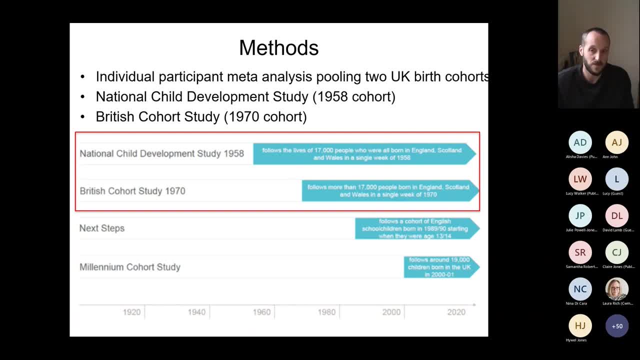 fact that they are managed by the same organization, the center for longitudinal studies, and that what that means is that there's some harmonization in terms of the assessments that they use and also there are set the harmonizations in terms of uh, the years at which items are. 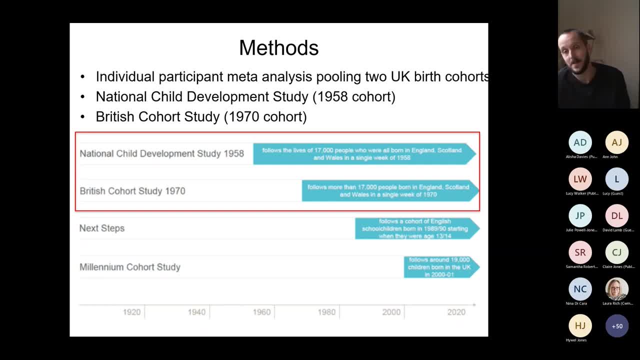 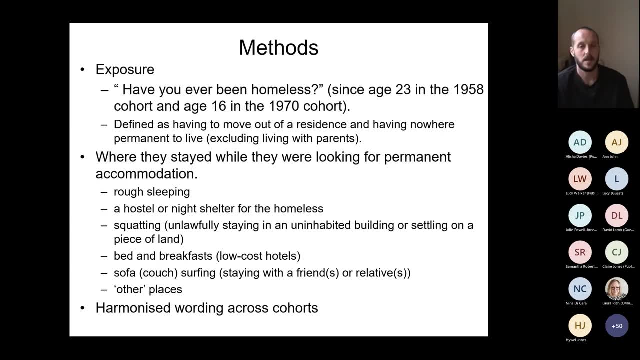 assessed. so in the year 2000 and recently in the pandemic, the same items were presented to people in these two different cohorts, which are of different ages. so the exposure in this study was a in terms of which diseases to use and um, so it was done in different genres. 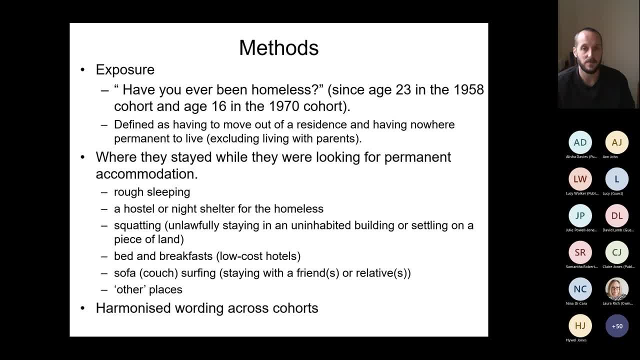 in the Institut surespace. the body was harder on the body was harder on the body. so we summarized the data often by interests. Bonus 3 has taken a factor of nine. split white and brown zone, which is a combination of n to small pinch rates and n to small. 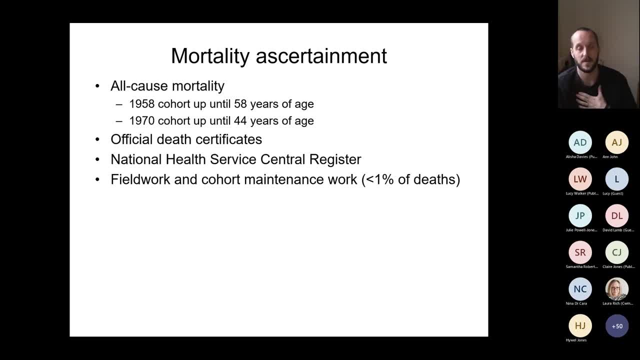 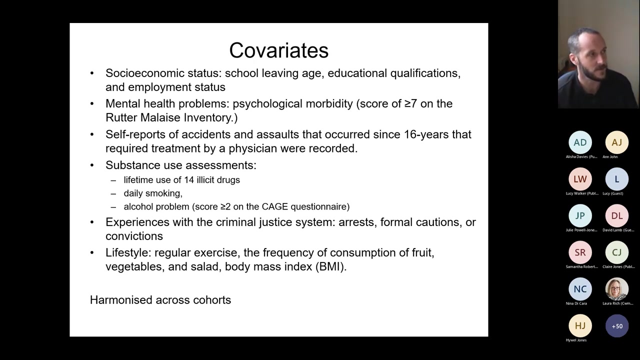 people were followed up. the outcome was all cause mortality and followed up until middle to old age across the two cohorts, and majority of those deaths were registered to the ons, the mortality file. but some are also mopped up through field work where people attract and follow-up studies in terms of covariates. so the good thing picking up on some of you know. 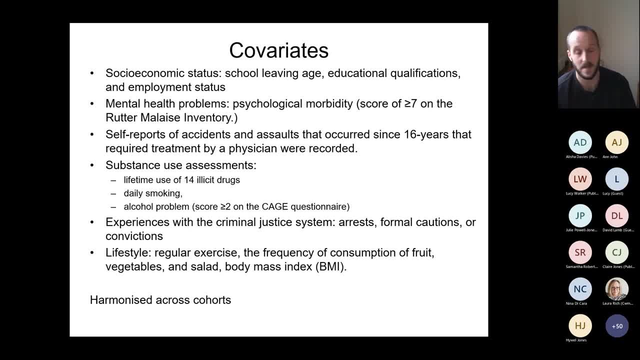 the points that i made. you know, the bad thing about cohort studies is we lose people, and the good thing about them, though, is that they're often what we call well described, so they have often really detailed individual level measures of potential confounding or mediating variables, so i've listed a few there that were we looked into, such as socioeconomic. 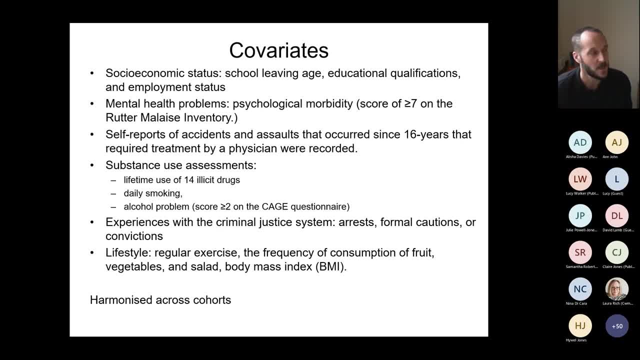 status: self-reported accidents, substance misuse. so you know, whereas in a, in record link data, you'll have information on. you know, uh, whether someone has a drug you misuse disorder? uh, here we've got assessments of. you know, the lifetime use of uh 14 different illicit drugs. 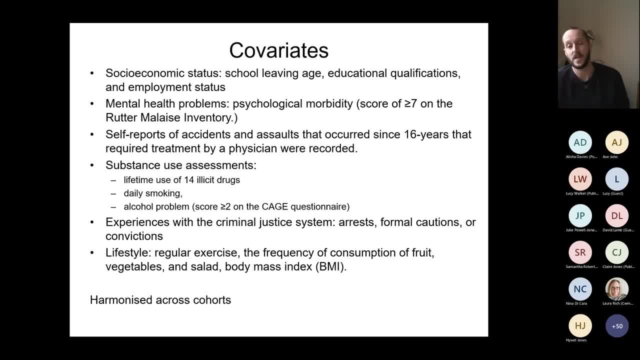 we've got information on daily smoking, as well as um screening of uh or for people for alcohol problems, and we also looked at the factors such as contacts with the criminal justice system and more broader lifestyle variables. i thought i should please- given it's an rss talk- talk a little. 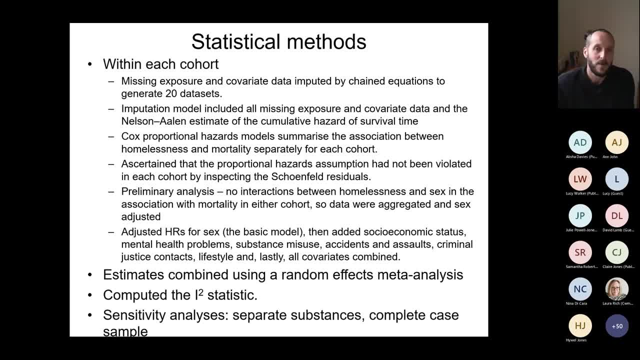 bit about statistical methods that we used. so um what we did within each cohort, we um we imputed exposure to covariate data, um we then did a proportional hazards analysis with it within each cohort, um adjusting for each set of covariates, and we looked at some of the assumption whether 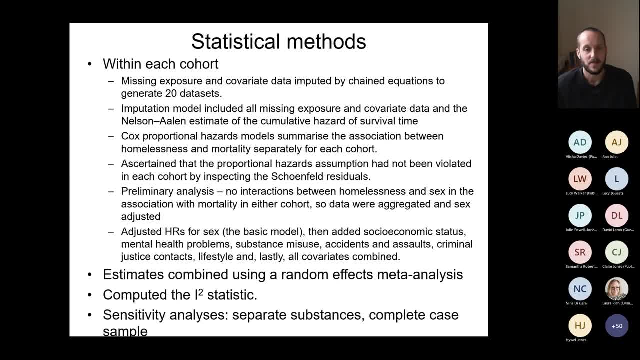 some of the assumptions of proportional hazards models have been violated, and did some preliminary analysis to see if there was any interaction between homelessness and sex. um, and then, as i just said, we adjusted for the hazard ratio, uh, for different sets of covariates. we then combined the result from the 58 and 70 whole in a random effects. 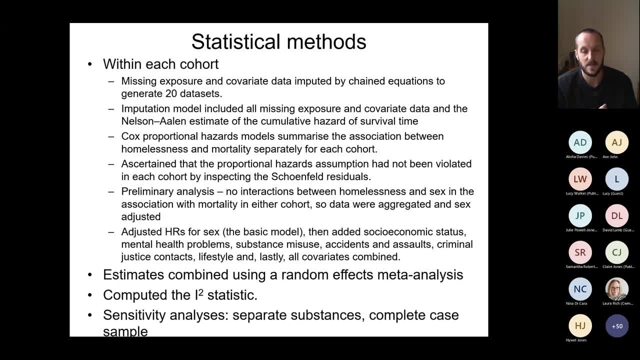 meta-analysis, looked at heterogeneity and did some sensitivity analysis looking at different substances. so some uh studies have found uh that particularly uh opiate use is much more common as a cause of death within homelessness populations. so we looked at opiates and we looked at uh, separated out opiates from other drugs and then looked at smoking and alcohol. 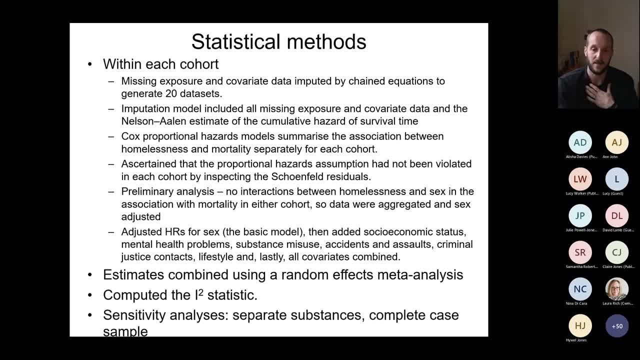 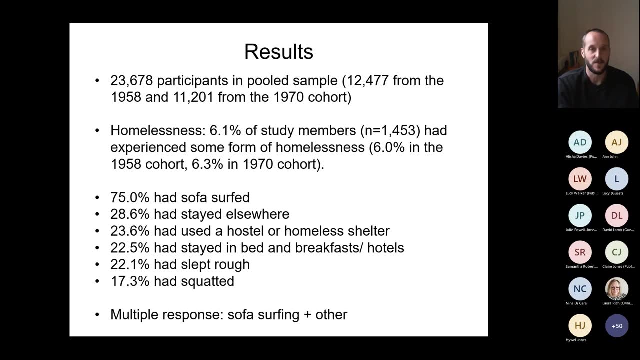 and also looked at um reran the analysis in a complete case sample, just in case. one is an assessment of any bias introduced by missing us. secondly, to see if anything gone awry with our imputation model. so in the pool analysis there were around about 23 and a half. 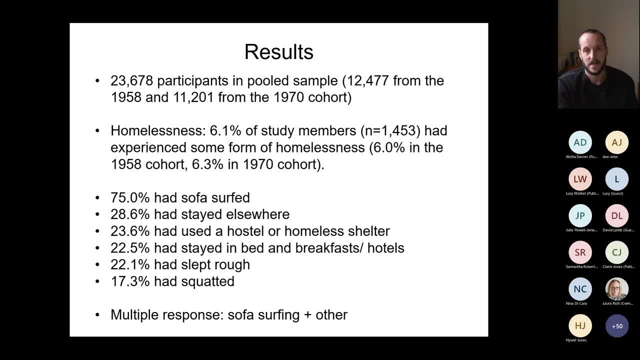 uh thousand participants and six point one percent said they'd ever been homeless. it was broadly comparable across both cohorts and nearly three quarters said they'd sofa surfed around. a third said they stayed elsewhere and then options of a hostile bread and breakfast use and sleeping rough around 20 and squatting was lower and people could. 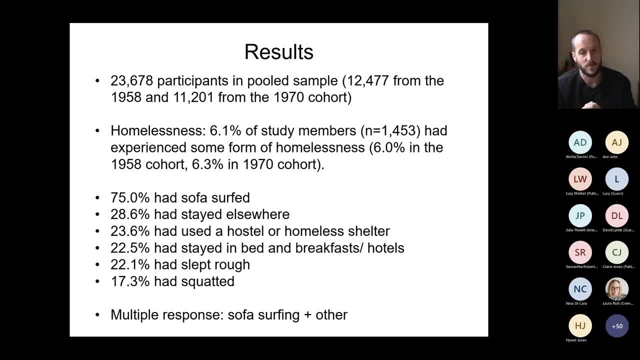 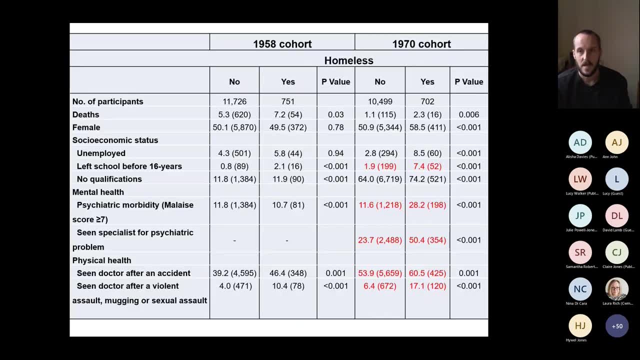 select more than one option. so the most common multiple response is people who had sofa surfed and, uh, stayed elsewhere or another place. this is a table showing for each cohort and differences between people who had said they'd ever been homeless or not, and in alignment with 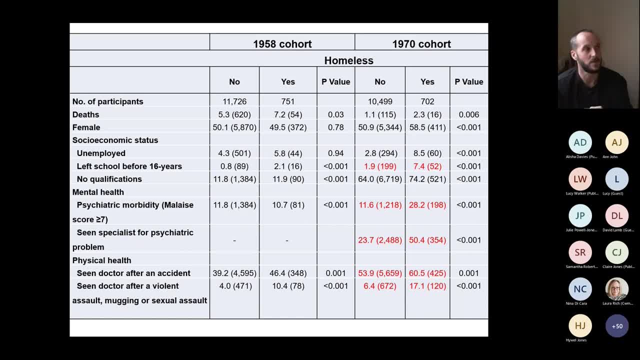 the, the data from previous cohorts and people reporting to um local authorities for assistance. we find great preponderance of socioeconomic disadvantage, mental health problems and also seen a doctor for an accident or a violent assault, mugging, a sexual assault in the homelessness group and the um never been homeless group. 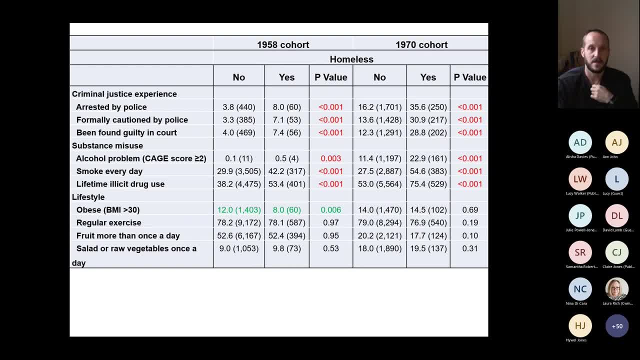 this is the day, uh, and i think this, as we would expect, the, the people who have been homeless are more likely to report contacts with the criminal justice system and report substance misuse. um, one thing i know i didn't know they are putting green is that in the 58 cohort we found more. 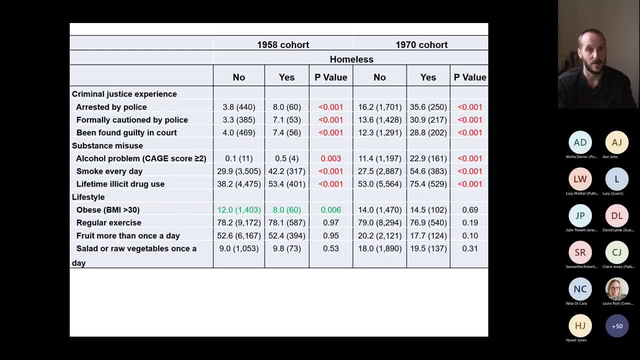 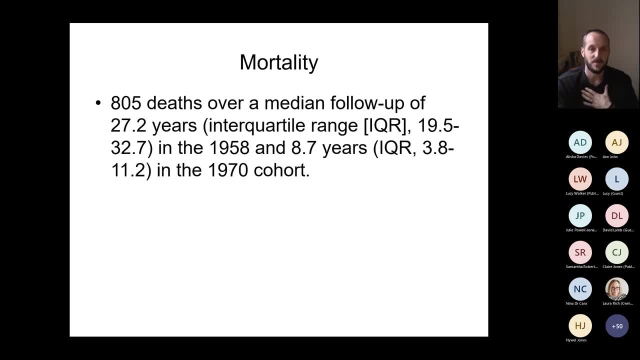 people who were obese in, who hadn't been homeless than who had been homeless. uh, we didn't find that in the 70 cohort mortality we had a 805 deaths. the follow-up was longer in the 58 cohort than the uh the 1970 cohort. 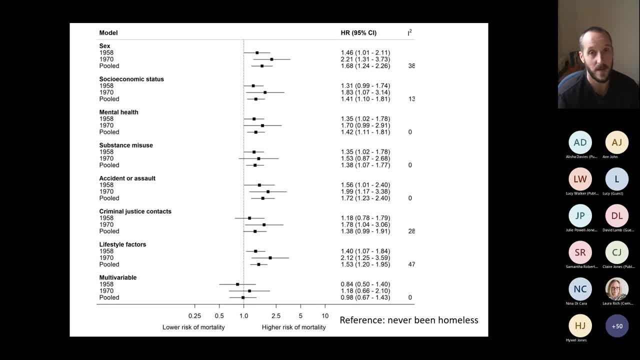 so this is a forest plot of um, comparing people who had ever been homeless to people who had not been, and what we're looking at is, for those who aren't familiar: if the lines are to the right of the dots, that indicates that there's an increased risk of death in the homeless than the uh never. 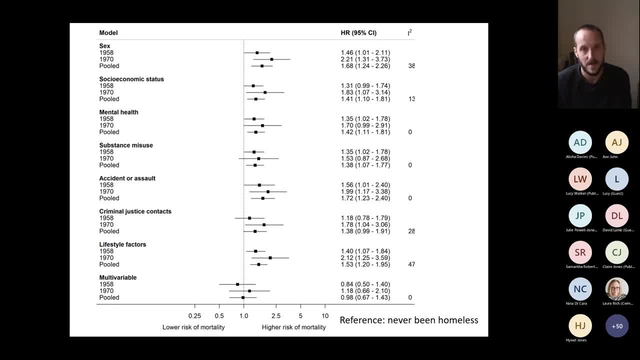 been homeless group um and what it roughly shows is that across the models that there is an increased risk of death in the um, the homelessness- than the never homelessness group, and that there was some moderate levels of attenuation after adjusting for socioeconomic status, mental health, the other sets of covariates. but 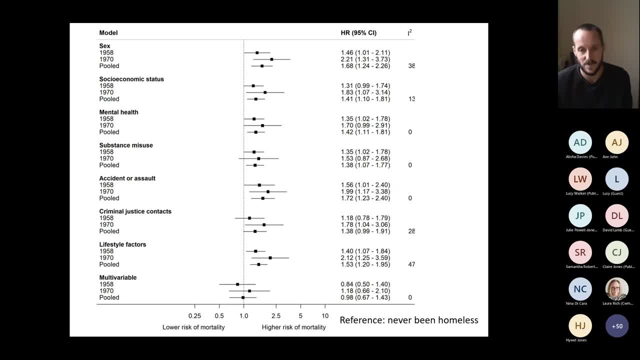 the. the association wasn't fully explained until we adjusted for them all in the multi-variable model at the bottom. and then the other thing i suppose i note here is that in the majority of models there there wasn't much evidence of heterogeneity between the two cohorts. 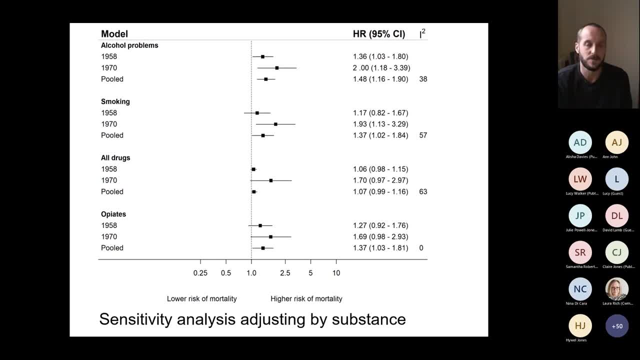 this is a sensitivity analysis where we broke down the substance misuse, uh group into uh the different substances and um. there isn't much difference in terms of the pattern of results for the pool um across alcohol, smoking and all drugs or opiates. there were other prevalence of opiates. 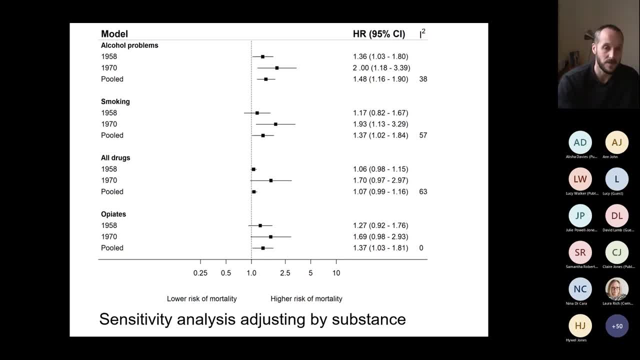 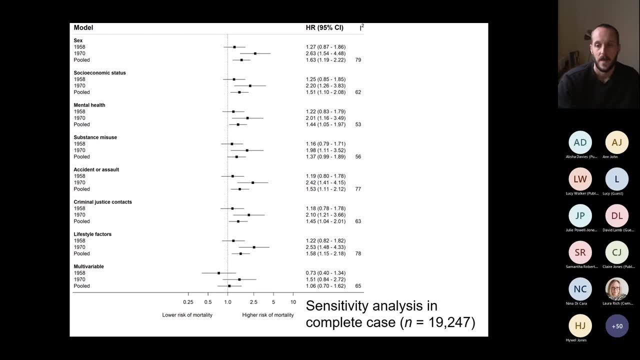 was low. it was around eight full higher in the homelessness than the not homelessness group, but that didn't seem to completely explain, um the increased risk for mortality. this is just the complete case results, so, um which ensure our we look at the case history and then we look at the 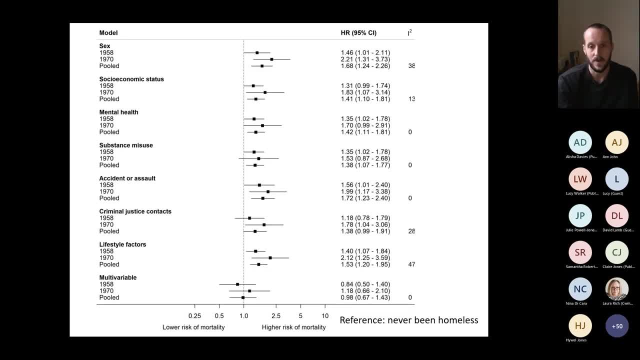 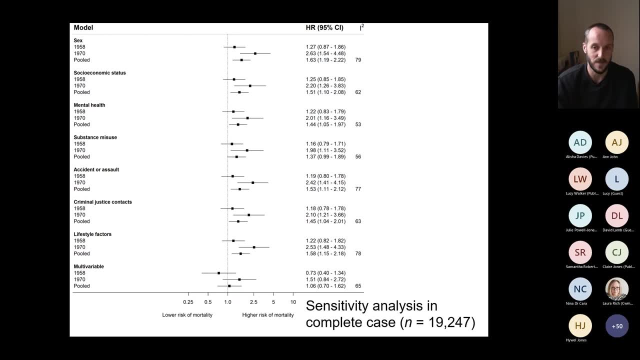 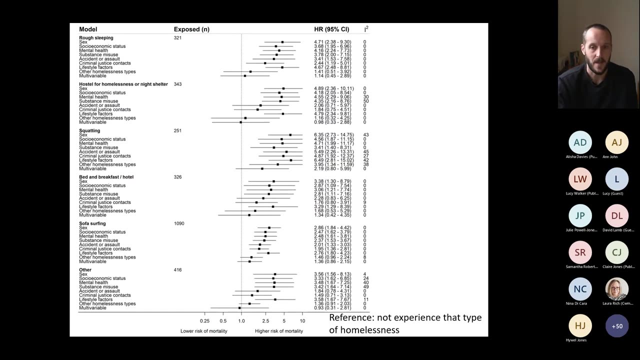 at that one there and we look at that one there. they're pretty much the same. so in the complete case analysis we had around we had 19 247 and in the imputed sample it was about 23 and a half thousand. so there was wasn't much difference there. so this is a busy slide, uh, but what it? 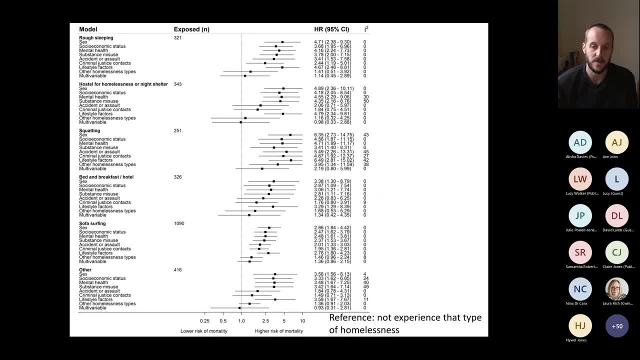 shows, is the same thing as the previous slide. this is in the computed sample and this is by different types of bonuses. so we're comparing here people who had reported rough sleeping comparison to those who had not, and and then, across the various uh adjustments going down the the kind of headline results are, is that the largest hazard ratios are pretty much as. 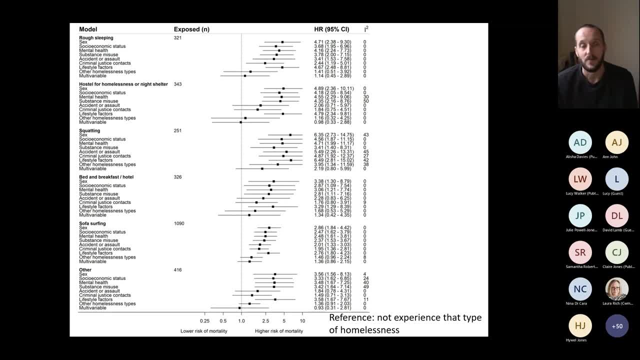 we expected in for those people who reported squatting, rough sleeping and staying in hostels. um hazard ratios were somewhat lower for bed and breakfast use and sofa surfing. nonetheless, in these larger groups, most prevalent, more prevalent groups, the risk of mortality was still elevated and then became explained as we kind of added more and more adjustments in the 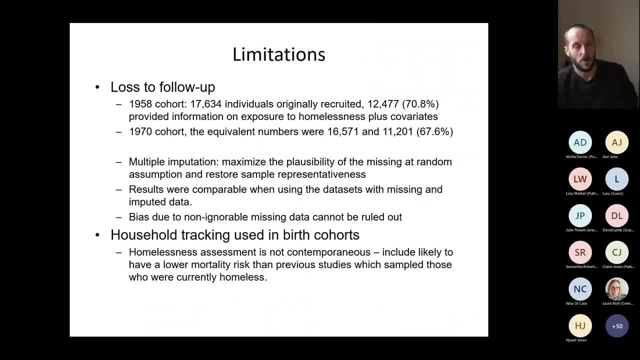 model. so in terms of limitations, so uh, in all cohort studies uh lost. the follow-up is a problem, um. so we included around 70 percent in the 58 and 67, 8 in the 1970 cohort of people who were originally recruited. we did impute the data uh and the daily results from the imputed in the complete case look comparable. 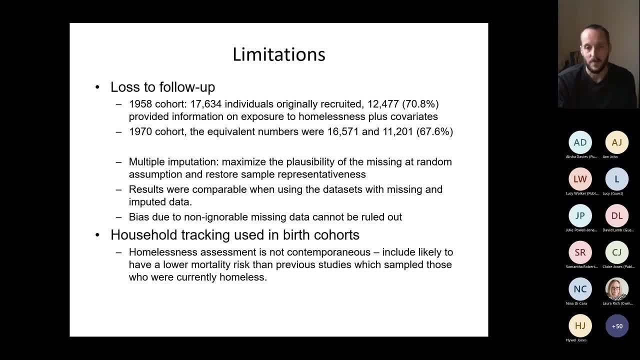 um, but there may be some sort of hidden, non-ignorable, missing data generating mechanism that that we can't completely rule out. and then another more important factor i would say is that, because these are household surveys, um to be included in these surveys, you had to be present um at a household, uh. 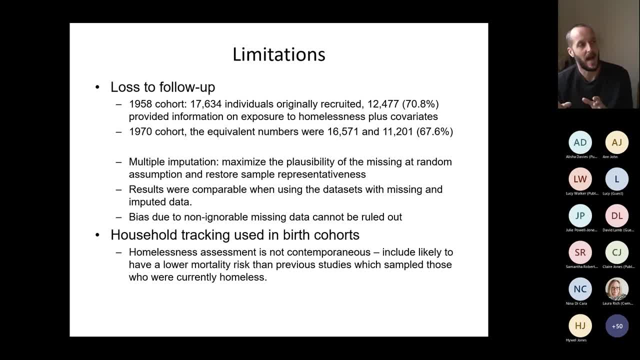 and so we're probably looking at people which how have been homeless, rather than people who are currently homeless, and that's very different to the groups of studies which look at rough sleeping and hostels in particular, which are nearly all for people who are currently homeless. so it's likely that in our study that the distribution of risk factors is probably a 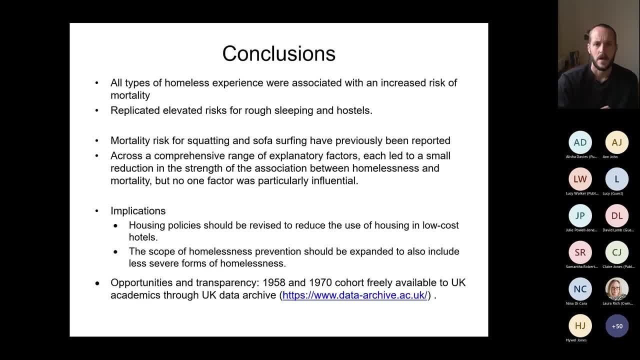 little bit lower than in those studies conclusions. i suppose the main conclusion is that we found that that across the full continuum of homelessness experience um mortality rates were elevated. we replicated the established risk for rough sleepers in a hotel and not people sleeping in hostels but in. we also found that for the larger group of people, so for surfing and 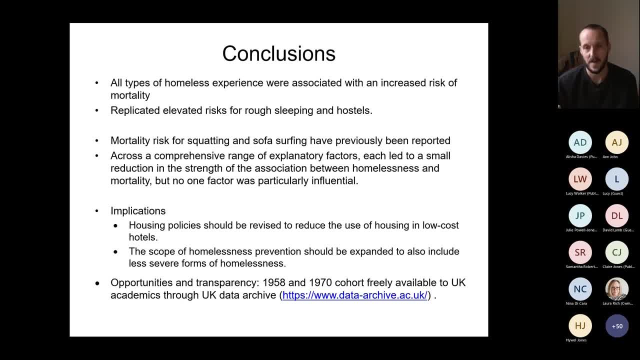 staying in bed and breakfasts, that elevated mortality which were elevated there as well, and, i suppose, more of an interesting thing that you know. often in my working cohorts we're looking to try and see if there are factors which explain these, and often we're looking for one. you know one thing we can pin our hopes on, because we can then intervene. 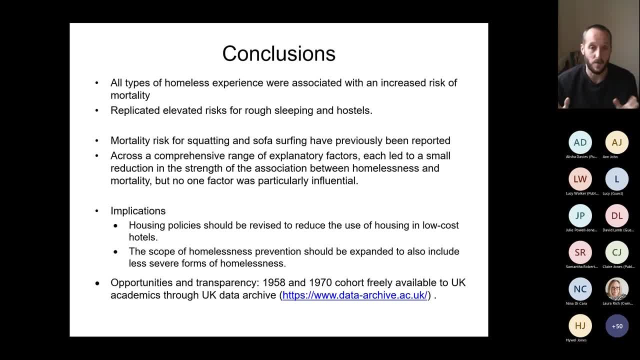 and do something about it. but we didn't really find there was one fact. it was more just across a range of explanatory factors, they all attenuated and explained a little bit of that increased mortality, but there wasn't one fact that it was particularly influential and in terms of 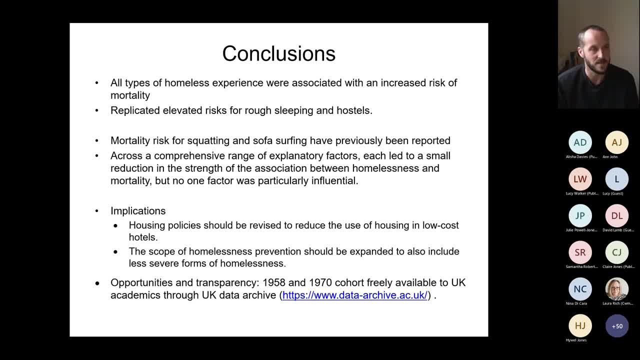 implications of the results. i suppose you know. what it does suggest is that, whilst you know it's good to move on people from rough sleeping hostels into low-cost hotels or bed and breakfast, that those people are still at increased risk, um, and that you know if we could move those into stable housing. that 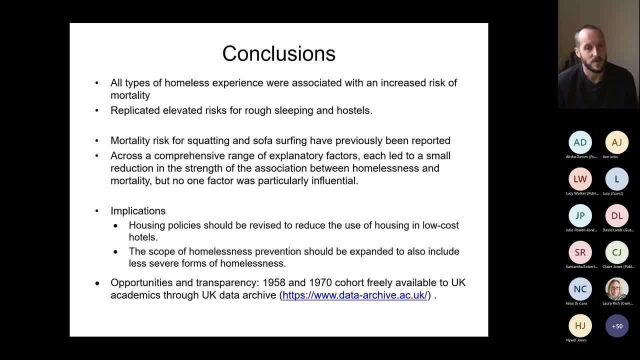 would be a better solution. um, the other thing, i suppose, is that the scope of homelessness prevention um really centers on those homeless, the hostel users and the rough sleepers, but what this result suggests is that there should be some sort of- uh, broad broadening of the scope of prevention and to include these less severe forms of sofa surfing and 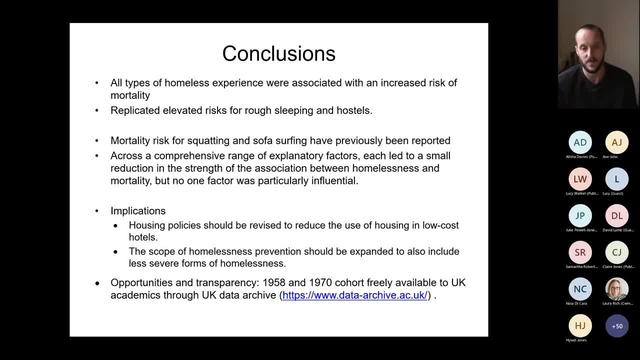 low-cost housing, low-cost like low-cost hotel or bed and breakfast use. and then the other thing i'd note is that, um, these data are freely available. so if you're a uk academic, you can download this data. you can seek to, you know, recreate our analysis if you wish. there's also 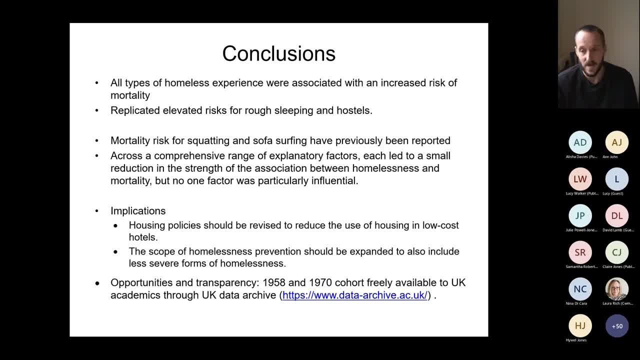 lots of weather. you know exposures and conveyors out there related to homelessness and other forms of social economic disadvantage that, um, you can analyze, and so if you know you're a junior researcher and you, you, you want like to access some data, i'd encourage you to look at the uk. 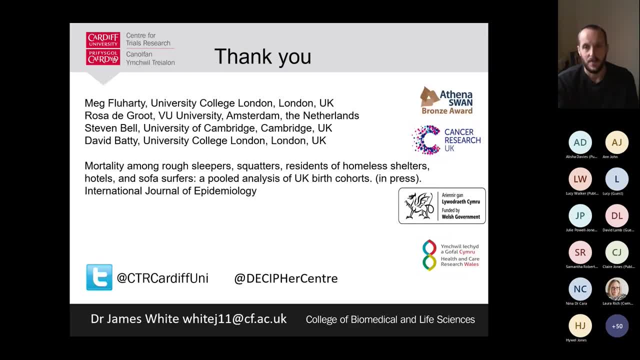 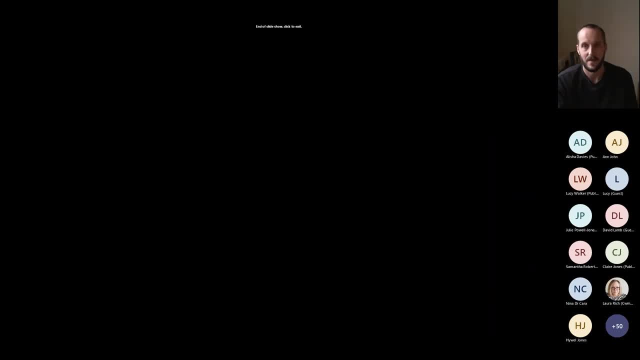 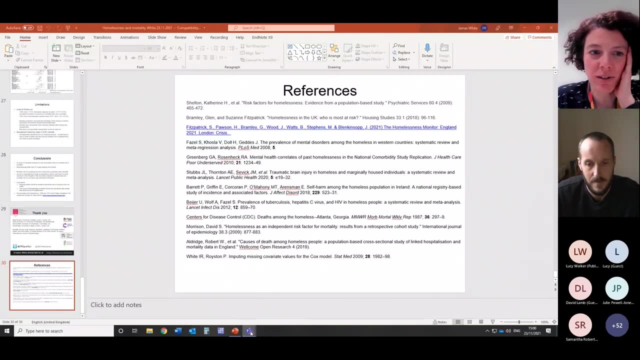 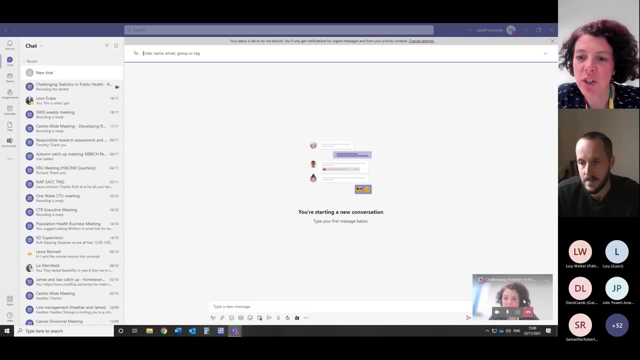 data archive and there my collaborators and the papers coming out soon in ij. hopefully there's my references. that's it, but very few are going to be on the internet, so i just want to let you know. thank you for your time. thank you very much, please, um. thank you very much for your time and i really 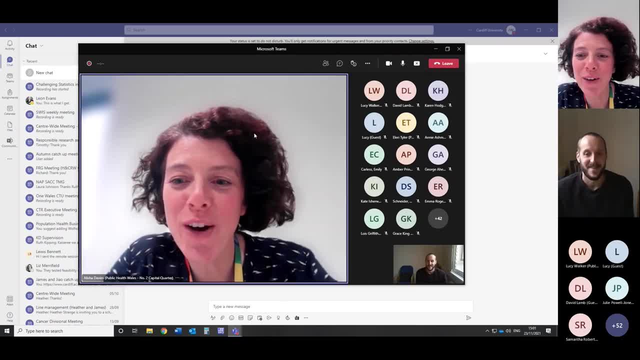 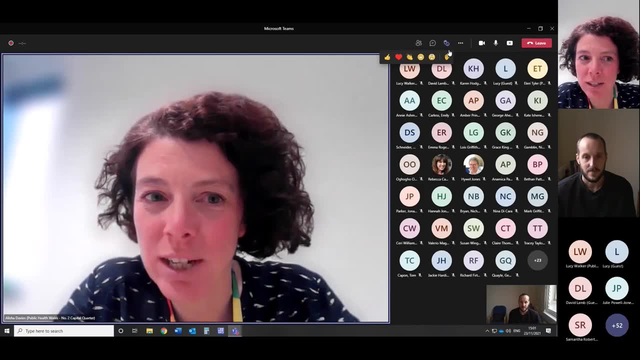 appreciate it, but i'm just going to turn this over to you and wait for the next one i'm going to take. i'm thinking i'm going to take one or two notes and then i'm going to just quickly see if i'm getting into the notes. yes, so let's see if i can get to welcome another. 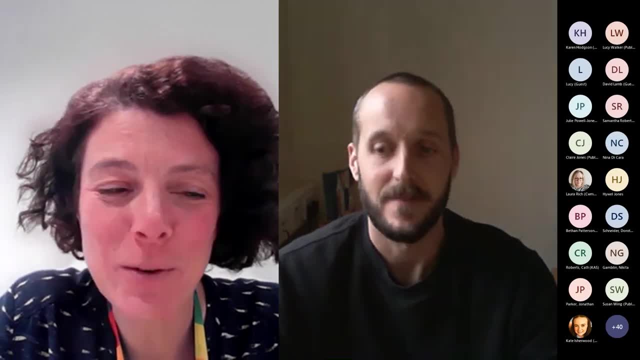 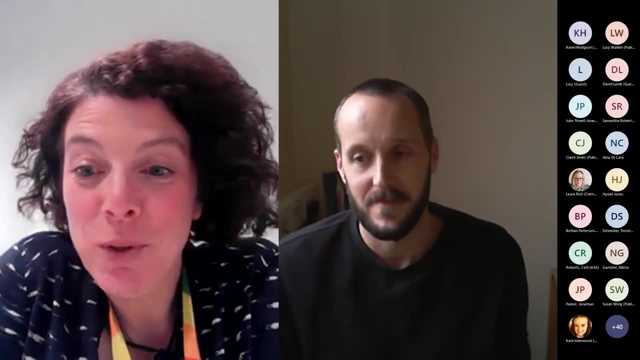 question that is coming in from the audience. i'm going to stop the recording here and let you answer that one. i think i'm looking at a request from jimmy cheong, who's going to come in soon. mute. um, thanks, james. um, what i was saying was that was fantastic, really comprehensive um. overview of 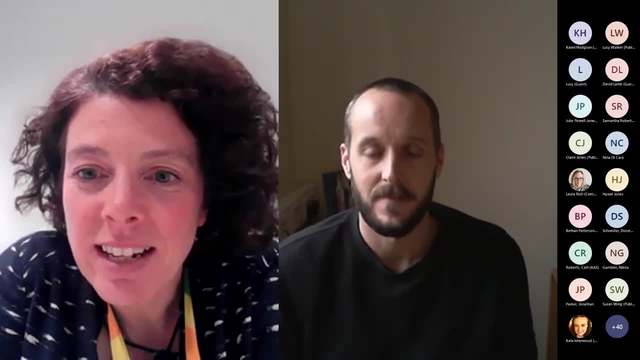 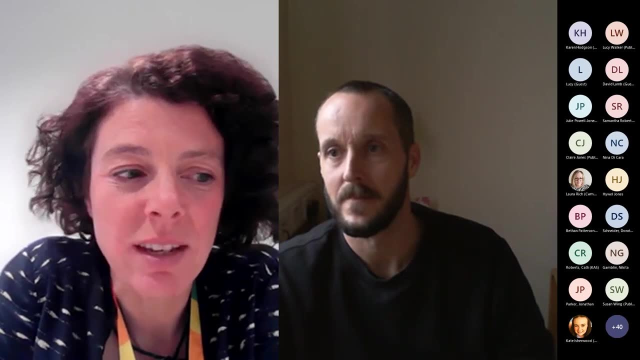 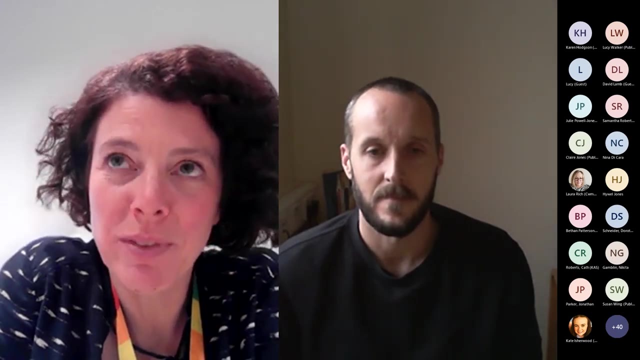 of homelessness, but also the social factors. um again, any questions to uh, drop them in the chat or pop your hand up and we can ask. um you can ask james. the other fascinating thing was, in those two cohorts, at very different times um, like one in the 50s and one in the 70s, the factors that 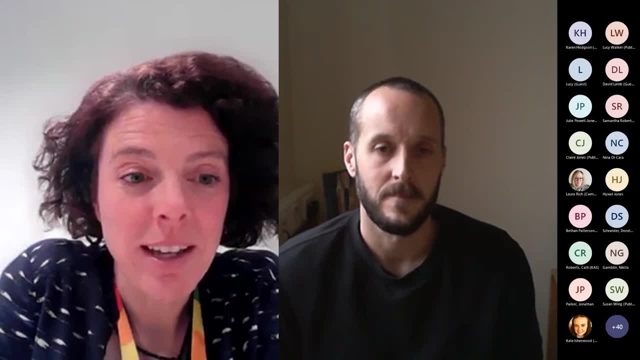 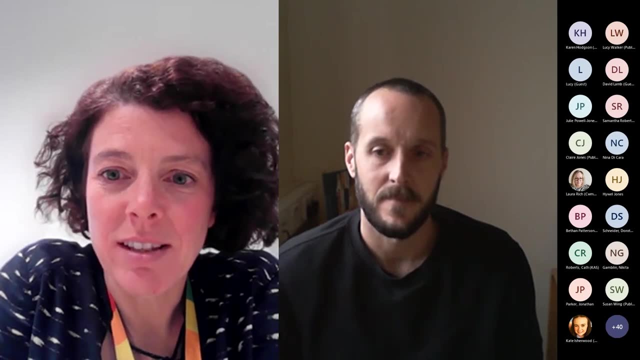 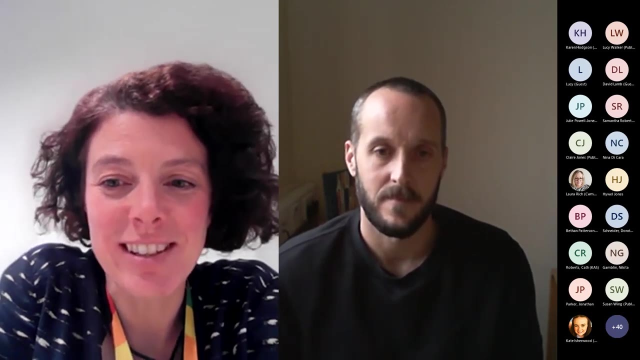 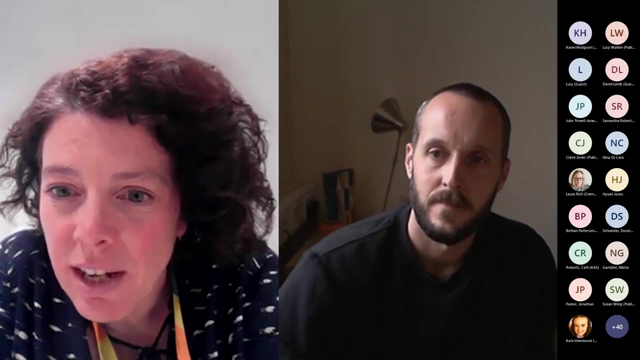 contribute or correlates with homelessness are all largely the same and if you did that again today, they're largely the same um, and it just highlights how difficult it is to really address some of the underlying socio and economic factors that are creating the conditions that are resulting in um, in homelessness. um, really, really good stuff um. 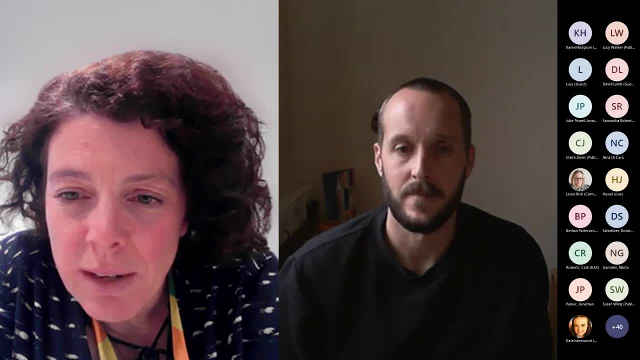 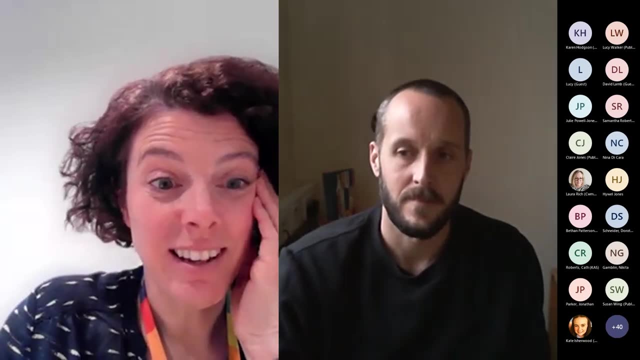 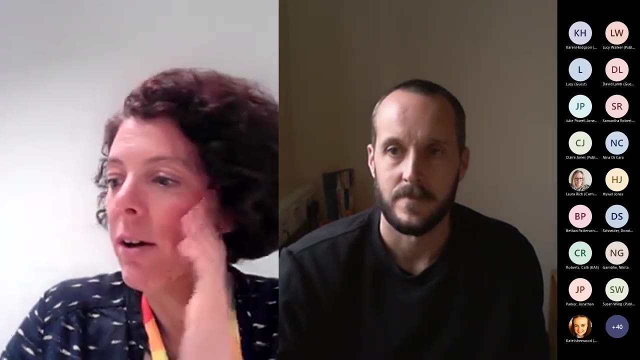 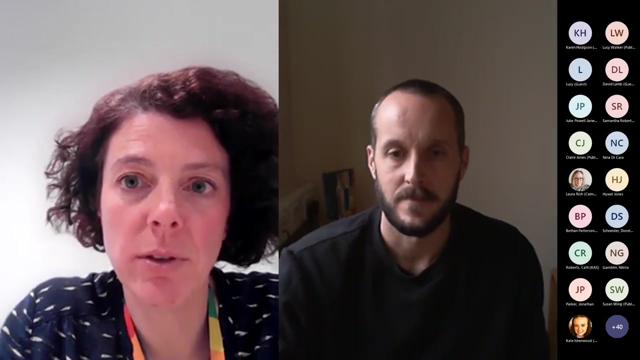 um, there's no questions for you, james. i think we've been. we've linked up- hopefully jow's linked up- with the work that she's been doing on homelessness as well, in um, in routine data as well too. so fantastic and um, uh and wonderful of the cohorts as well, to be freely available for those of you that um are really. 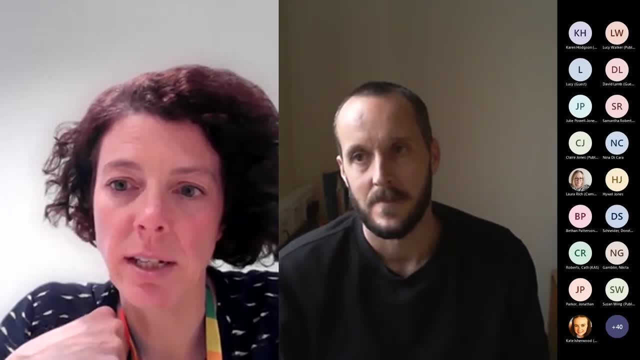 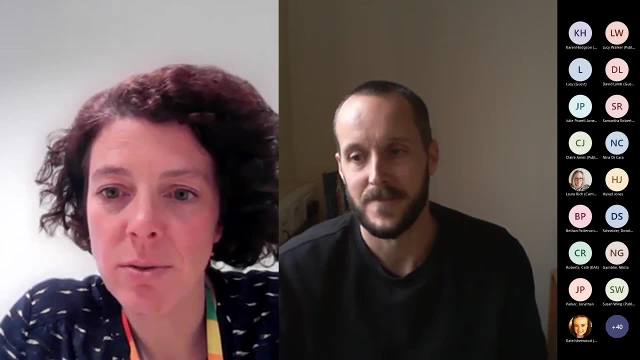 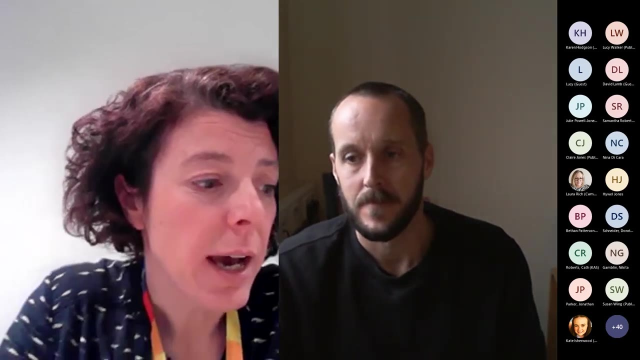 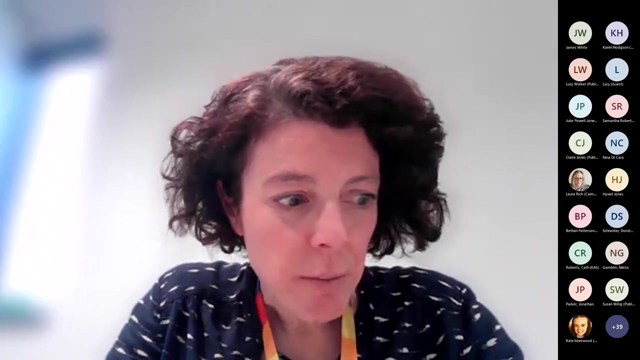 interested in getting to getting to grips with that type of data if you haven't done that before, so let's see. fantastic. thank you ever so much, james. if there's any questions, um, we're going to move on to our third speaker for this afternoon, um, which is, uh, claudia responica. hopefully claudia's here, and 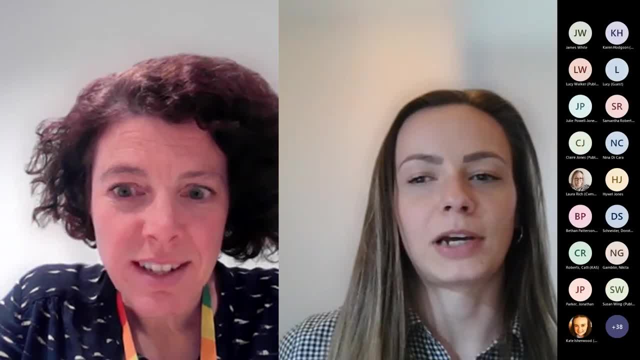 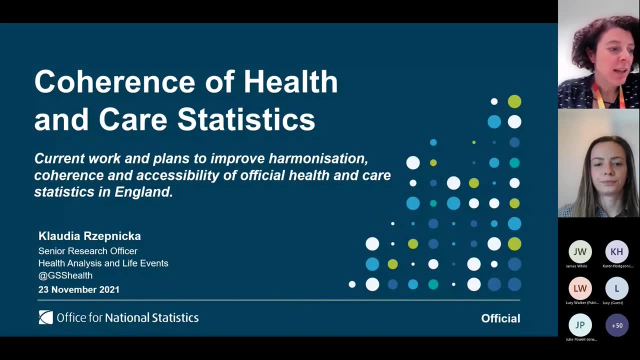 from ons. lovely hello. welcome, claudia, thank you. thank you for joining us. um uh, claudia's working within um ons and focusing on the coherence- um, oh, there we go- coherence of health and care and statistics. so, claudia, over to you, really looking forward to this as well. there we go. 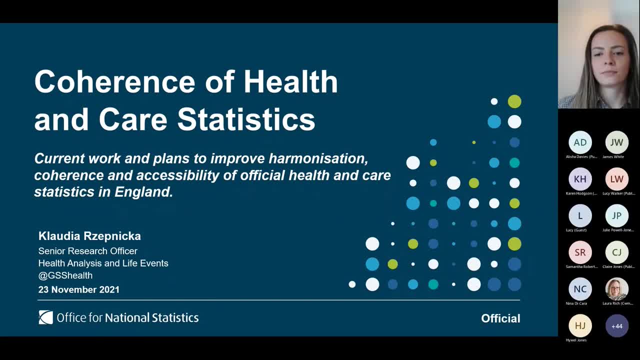 um, can you see the slides okay? um, yes, that's fantastic, amazing. yeah, thank you for introducing me and, yes, thank you all for joining, and, uh, so i'll be talking about coherence of health and care statistics, something a little bit different than the two previous conversations, and i'm going to 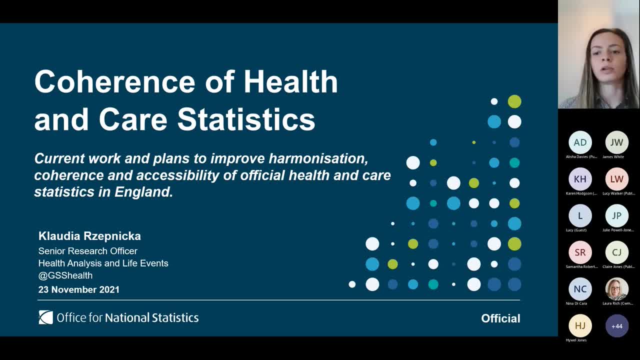 talk a little bit more about the two previous conversations. uh, or presentations, sorry, as we will be looking at the challenging nature of health and care statistics in england. um, i'll talk you through our current work and our plans to improve harmonization, coherence and accessibility of 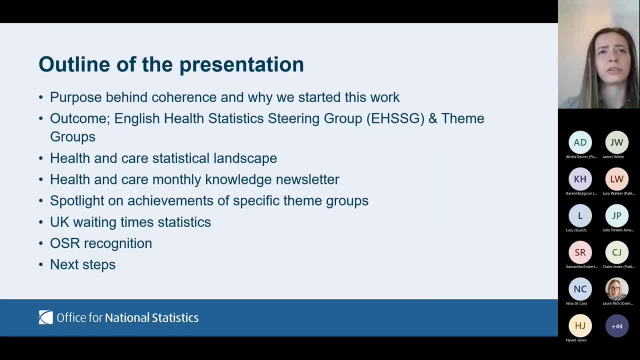